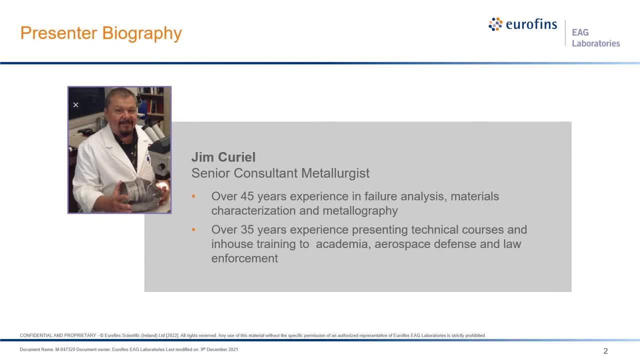 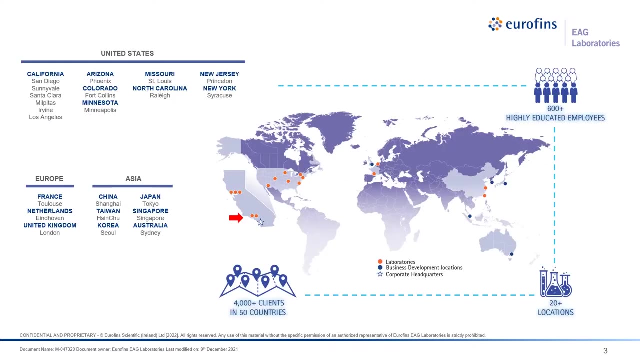 of experience in failure analysis, materials characterization and metallography and over 35 years in teaching, offering technical courses, in-house training for academia, aerospace, and defense and law enforcement. So a little bit about EAG Eurofence Company. 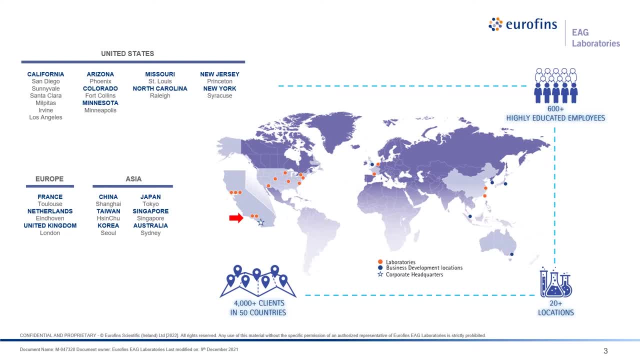 Eurofence has, for EAG actually has 600 plus highly educated employees in about 20 locations around the world, And EAG was established back in 1978 with an expertise of dealing with highly sophisticated, state-of-the-art technology and the staff that can apply that technology to your 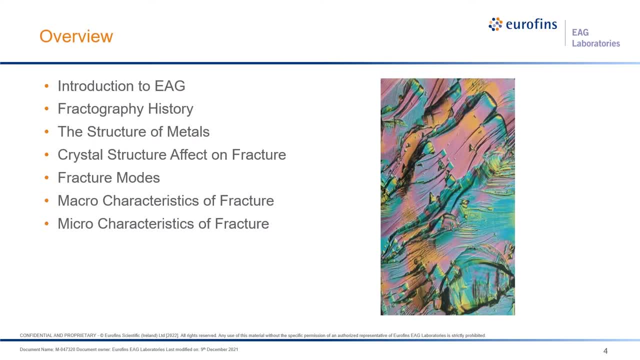 problem-solving needs. So what are we going to discuss today? Well, we'll talk briefly about the history of fractography. You know it's not necessarily something new. We'll discuss briefly the structure of metals. We need to have a fundamental understanding of what is a metal and how is it comprised. 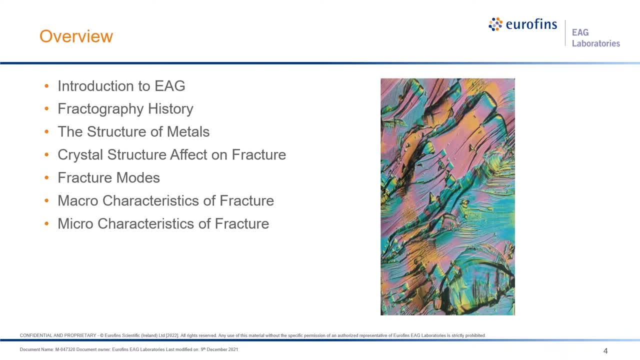 We'll look at the crystal structure and the effects of crystals on fracture, And then we'll talk fracture modes. We'll talk macro characteristics- Those are the characteristics that can be resolved with the naked eye or very low magnification- And then we'll look at 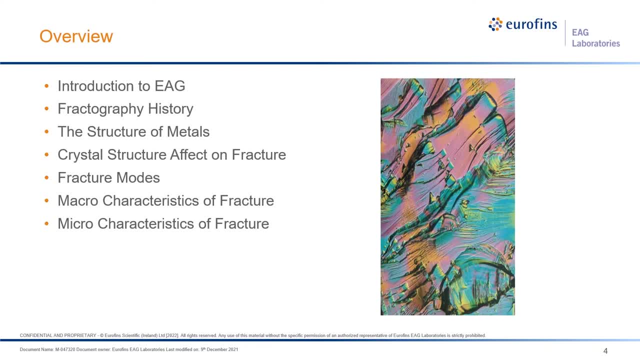 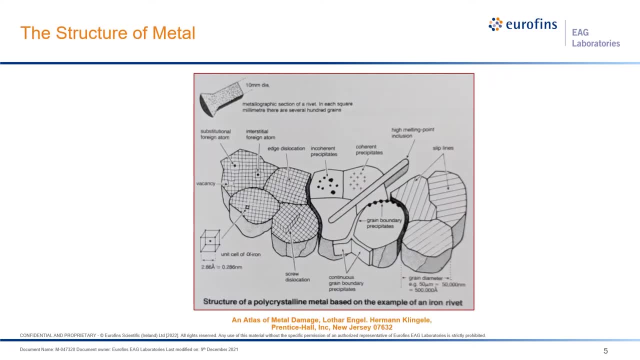 the micro characteristics, which do require a higher magnification and sometimes electron optics in order to resolve features. So the structure of metal. This is a very, very informative treatment of what is going on in metal. It's a very, very important part of what is going on in metal and I'm going to talk a little bit more about that in a moment. 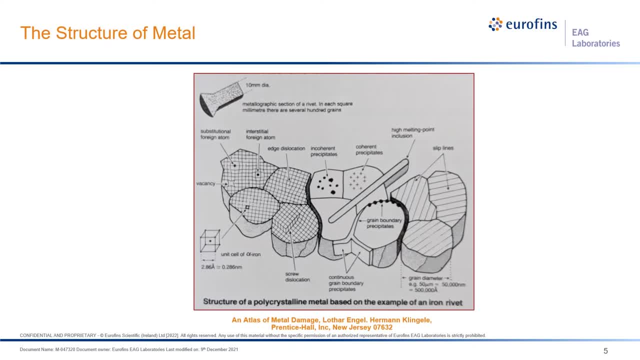 The structure of metal is a very, very informative treatment of what is going on in metal. It's a very, very informative treatment of what is going on in metal. going on in metal Now. first off, I need to clarify something that I hear all the time. People often 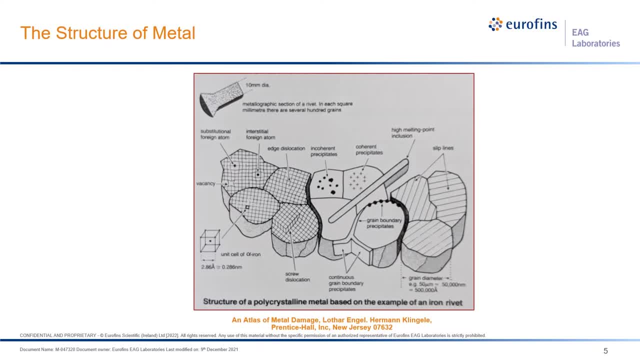 refer to grain structure as crystal structure, and crystals make up grains, so they shouldn't be used interchangeably. As we can see here, this is a unit cell of alpha iron, plain old iron, ferrite, and we have a grain here, and that grain is actually comprised of thousands, millions, you know. 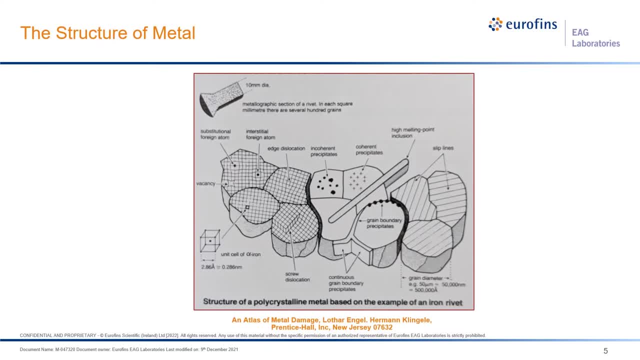 a lot of crystals Within that crystal structure. when you combine these cells, we then develop what is called a crystal lattice. We see that we have substitutional foreign atoms, we have interstitial atoms, We have dislocations, screw dislocations. Now, what are these dislocations? Well, basically dislocations. 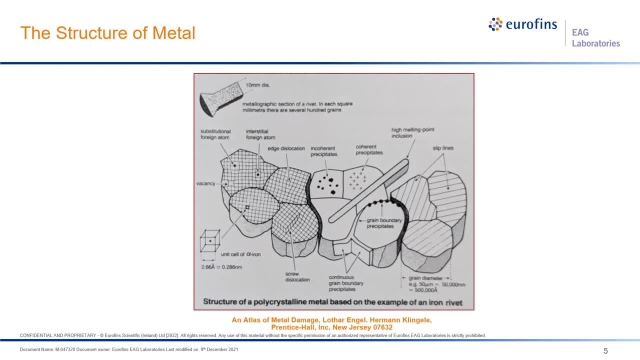 are flaws in the lattice structure, and the whole idea of having material that is easily deformed is to allow the crystals to rearrange themselves, for the atoms to rearrange themselves, and if they do not have that mobility then the material will act brittle. All of this over here is more for tomorrow's lecture, which is: 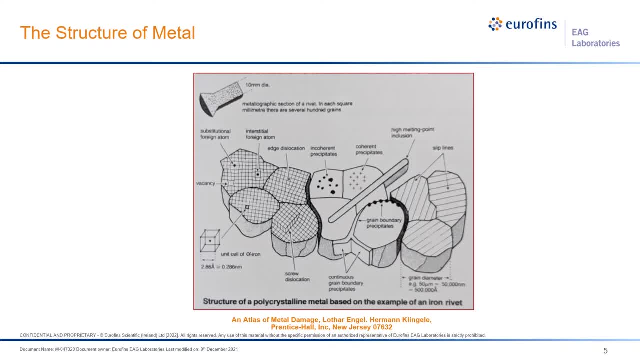 the metallography. but it does come into play because incoherent precipitates- those precipitates that do not go into solution- will affect what the fracture surface looks like. Coherent precipitates are precipitates that do go into solution, and these may or may not be a solution. 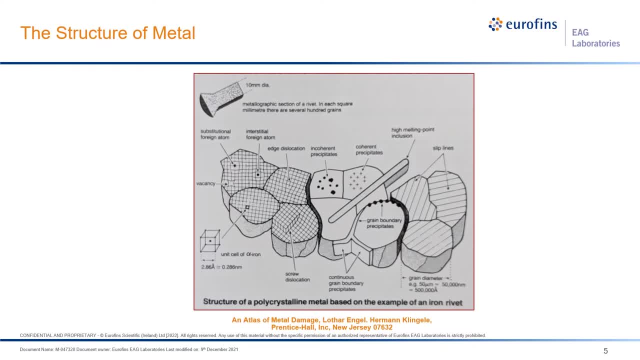 However, sometimes these are more benign High melting point inclusions and other artifacts We will see in fractures. Grain boundary precipitates are also important players. Grain boundaries are arguably the strongest part of the grain, so if we have precipitates along that grain boundary, that 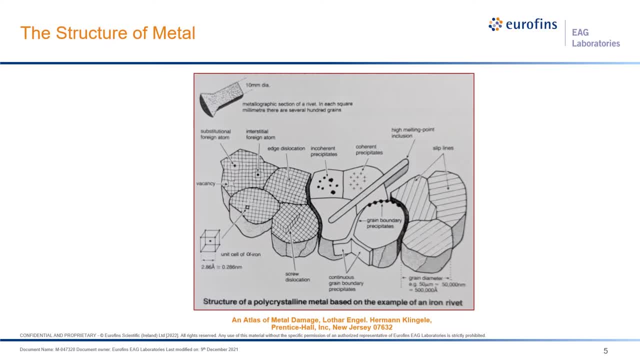 is going to inhibit what we call slip. you know, for example, if we have three rows of building blocks one on top of the other, and we take that center row and we move it left to right, it should slip very nicely along that axis. that's your slip plane. if we offset that center row by, oh, roughly half a. 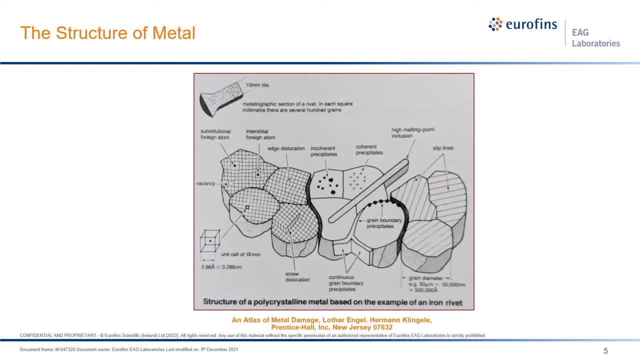 a building block and we try to do the same motion vertically, we are not going to be successful. we're going to fracture. and that is because that slip plane is being blocked. and that's what these guys do. these grain boundaries precipitates, they inhibit slip and they take a normally ductile 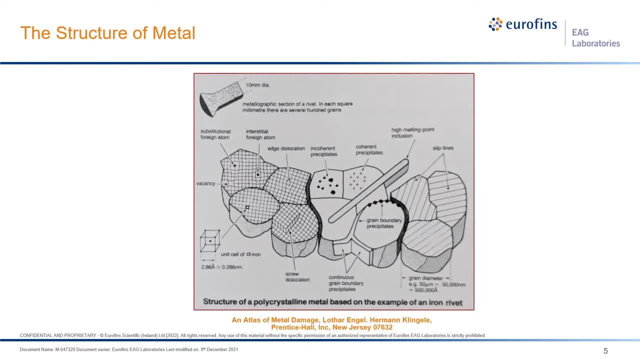 material and make it act brittle. this continuous grain boundary precipitates same same effect, but they can even be more insidious, because oftentimes these continuous films could be another metal. for example, you can have copper intrusion into iron. well, you have the mechanical properties of iron, which was designated for that application. and now what are you doing? 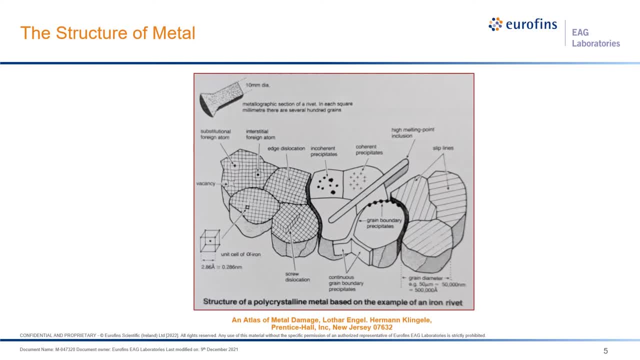 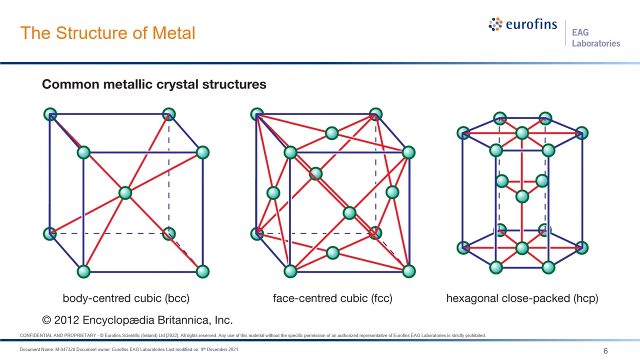 well you're. you're gluing the grains together with copper, so your mechanical properties have been diminished to that of the copper. so the microstructural details are very important in the study of fractures. now the most common crystal structures that we have for metallurgy are these three. there's many. 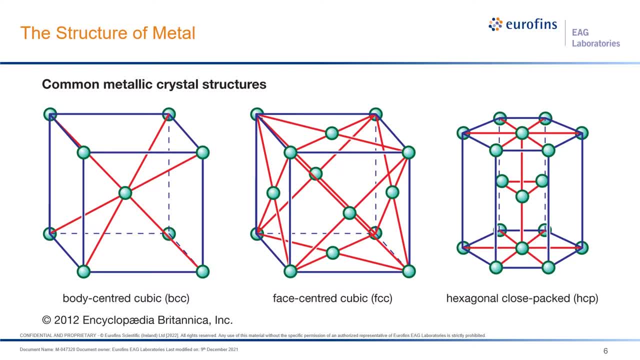 others, but these are the most prominent. we have body centered cubic, face centered cubic and hexagonal closed packed. now each one of these will have different properties and different responses to fracture. remember it's all about mobility and the ability of the slip system to be active. if we look at body center cubic here we see that we have very nice spacing here. 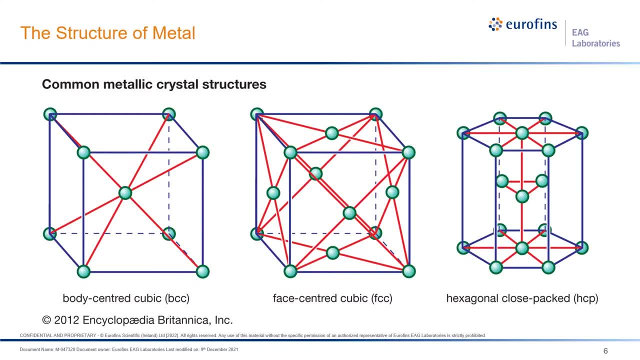 if we look at hexagonal- closed packed- we do not. it's a tight structure. as you can see, the name implies it's closed pack. this structure has room to move. this structure doesn't. this will exhibit ductility, malleability and this one will be limited in that area. face center cubic also. 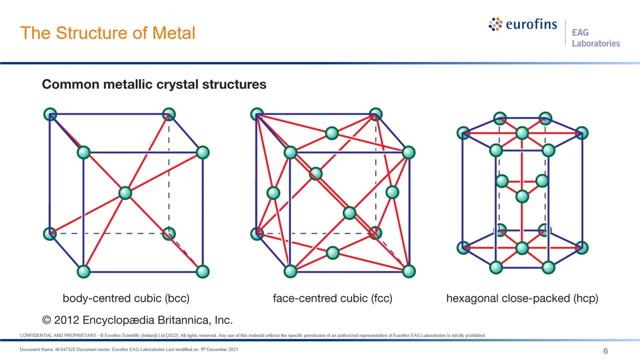 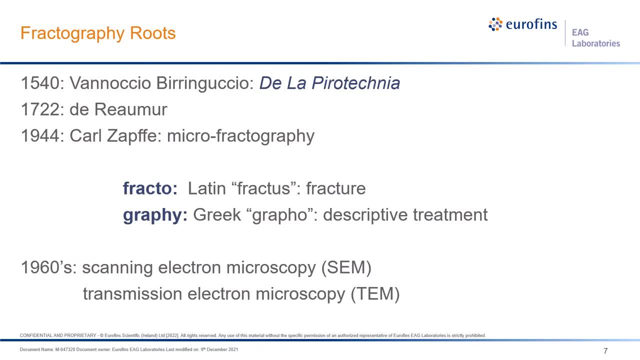 has a fair amount of ductility and malleability, but along different axes. so where did this all start? well, back in the 1540 ad Venocchio Beranguccio wrote de la productivity and in essence, he was looking at a way to perform quality control on copper. 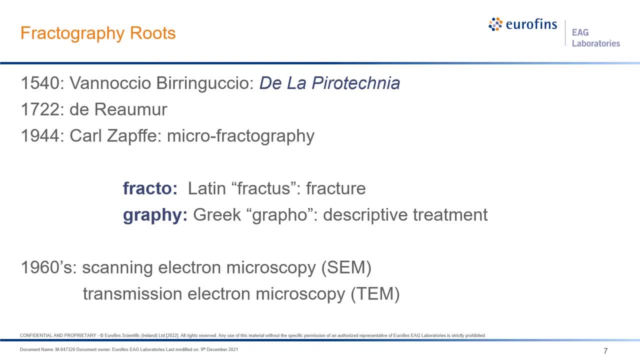 alloys. and then, a long time later, 1722, de remyrer came along and did some fantastic work in fracture and uh, illustrating, created a book- and actually they were hand-carved, the illustrations- and he came up with seven different classifications of fracture, ranging from woody to mirror-like. It wasn't until 1944. 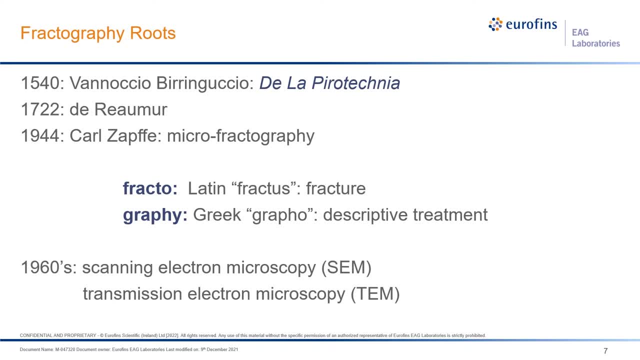 that Carl Zapfick actually coined the term micro-fractography. Up until that point, everything was pretty much dealing with the macroscopic world, that which can be resolved with the naked eye. Fractography is fractal, which is Latin for fractus, which is fracture. 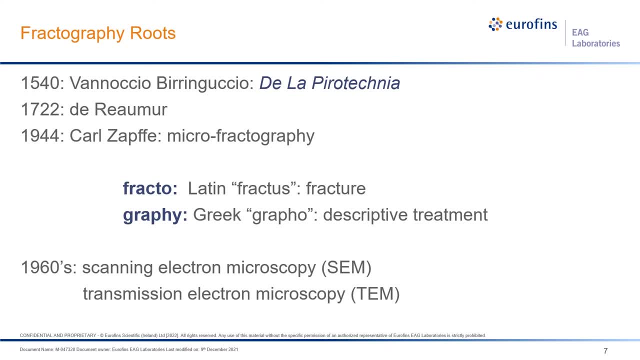 and graphy is of course Greek for graphal, which is a descriptive treatment. And then revolution began. 1960s. That's when the scanning electron microscope came into play and the transmission electron microscope. And at that point, 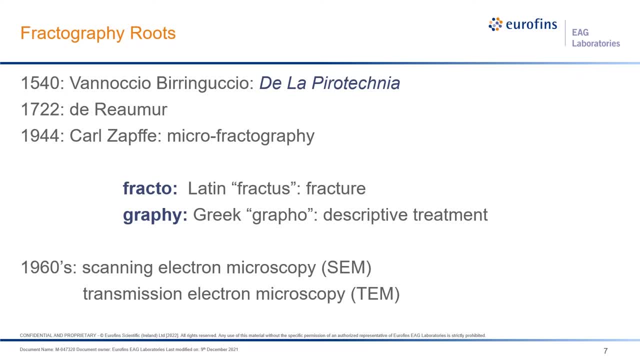 we had the ability to study the microscopic world and actually look at fractures and understand what was going on at the microscopic level. One of the problems we have with light optics is, of course, depth of field. You cannot resolve areas on various planes, separate planes. 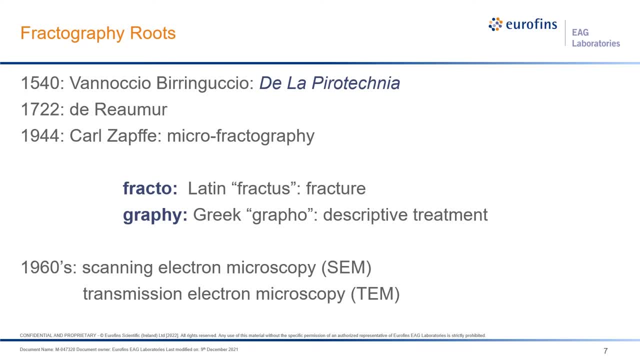 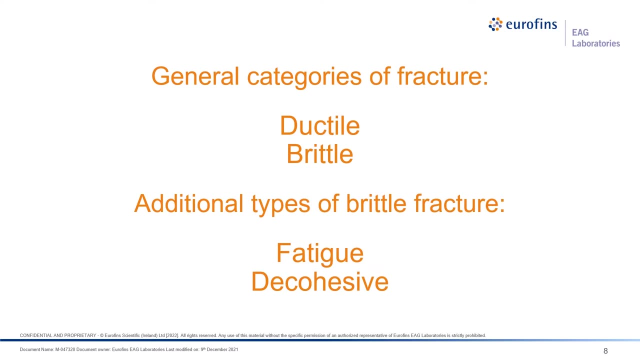 in focus at once. The SEM, the scanning electron microscope, does allow you to do that very nicely. So the SEM became one of the key players in fractography. So the types of fracture: Well, we have two primary categories. We have ductal fracture. 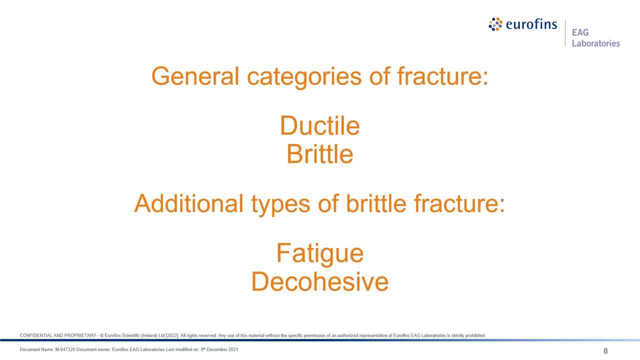 we have brittle fracture And then additionally we have two other types of brittle fracture because they exhibit brittle features. We have fatigue and we have decohistography, so we can be very, very sensitive to those perspectives. And then also the funniness of 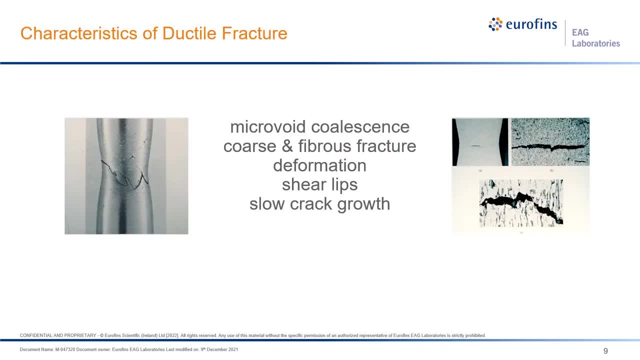 the rupture in the ductal material. When you look at a fracture, the structure of the rupture. we have three types of fractures, either in a tendril or in a ductal material, And the transfer of the rupture to the ductal material, as I said, depends on the site. 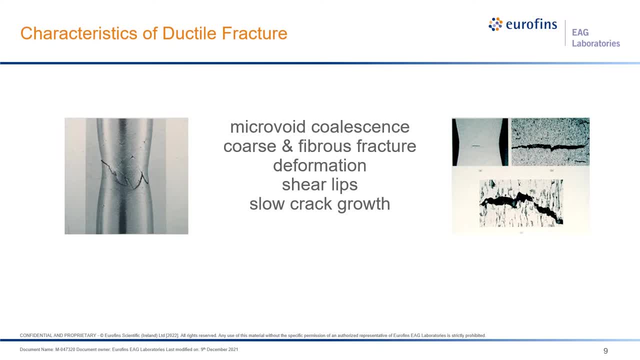 on the structure of the ductal material. You can see the structure on the left And then you might find holes on the surface. the sysloquine, You can see the structure on the left- hasn't been pulled, that the sides are parallel and flaw-free and we now apply an axial load. 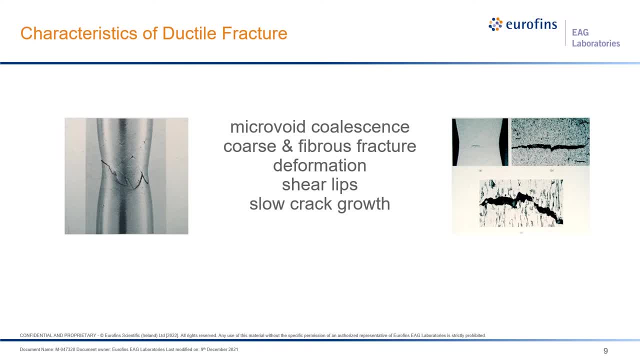 right down through the center. there, then the stress will be concentrated at a tri-axial stress concentration. in the center We will have a parallel plane and, I'm sorry, a perpendicular plane which is at right angles to the applied stress, and then we will have these 45-degree. 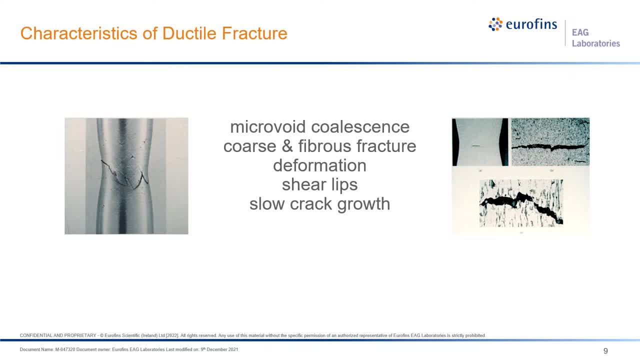 shear planes here on opposite sides or all the way around. When we continue to deform and apply stress, what will happen is the ductile material will actually pull away from microparticulates, secondary phase particles, inclusions etc. and as they do this, they form a minute separation around that particle, which assumes the same size. 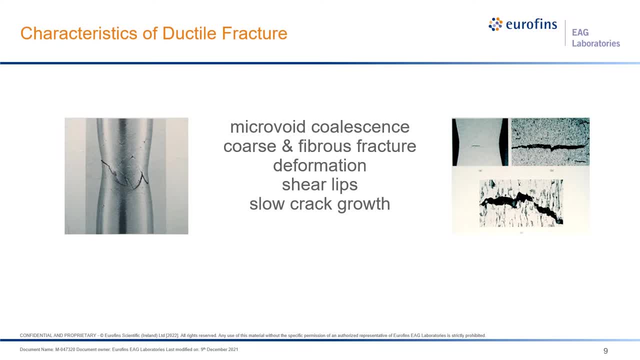 and shape of that particle, and with continued loading it pulls away and eventually we see them form a tear along that stress line there in the center. This one's slightly offset and that is when the microvoids coalesce. Well, now, in essence, we have a hollow sample. same load is being applied, so we start to reduce. 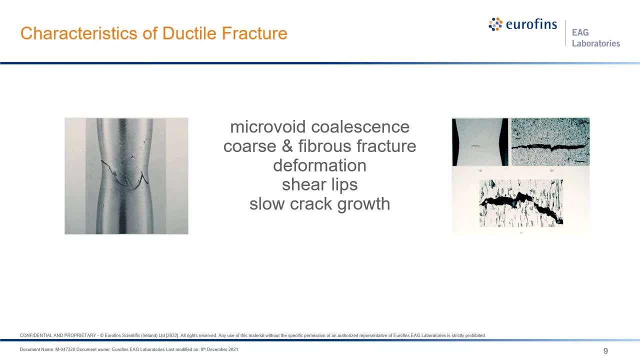 an area and that's when we see the necking here and we begin to deform and we begin to shear along these 45-degree shear planes until it finally ruptures. and when that occurs we have a 45-degree shear lip that is around the circular plane, and that's when we see the necking. 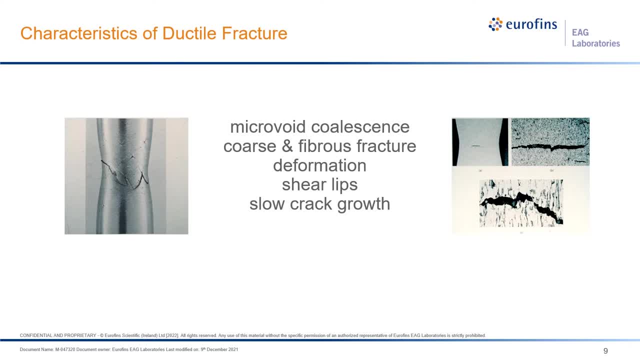 in the center, and that's when we see the wide circumference and a flat bottom. so in essence, it looks like a giant crater with a 45-degree shear plane surrounding that. The other features that are important for ductile are that it is a coarse, fibrous fracture. 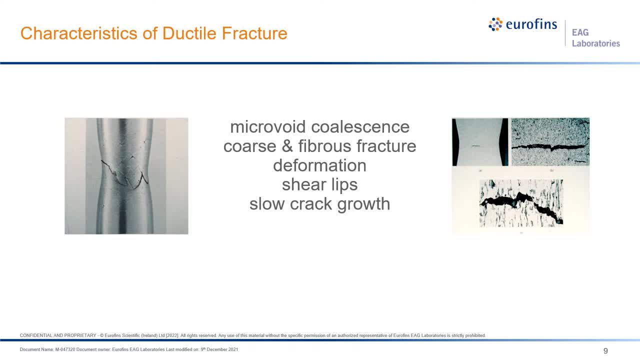 there's a lot of deformation. the shear lips are key and it tends to be a slow crack growth process. You know cracks can propagate at the speed of sound. Normally it doesn't. The interesting thing here I'd like to reinforce is shear lips. 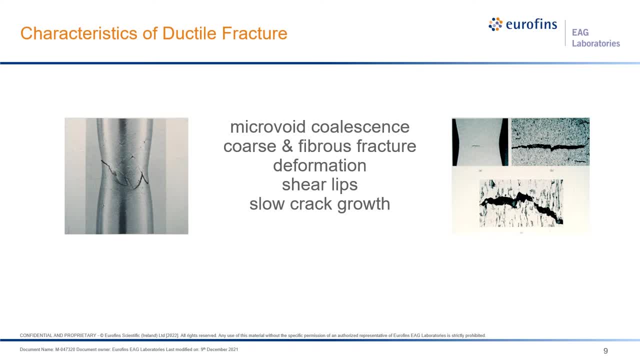 In the process of microvoid coalescence we saw that it was the point of final separation. was that shear lip In fractures, oftentimes fatigue fractures but any overload fractures of ductal materials or ductal acting materials, the shear lip will indicate the final point of separation. 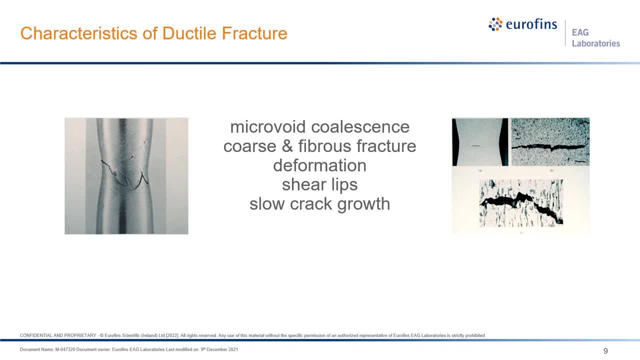 So if you resolve a shear lip, if you can see this 45-degree feature on the surface, chances are, if you look opposite, you'll find your origin. So it's very important to use shear lips in determining crack growth direction. 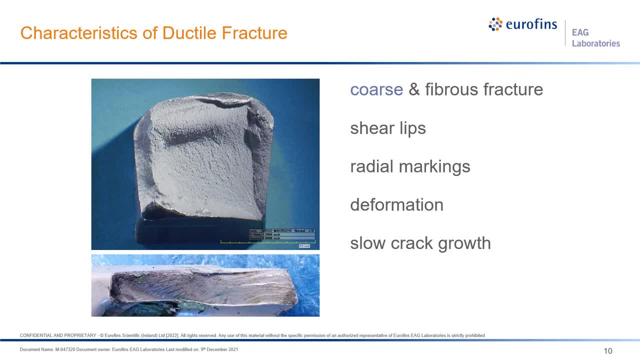 So what do we have here? Well, we have two examples of ductal fracture. In one instance, we have a solid cross Solid cross member And if you look very closely, you can see a repeating pattern radiating out from a point. 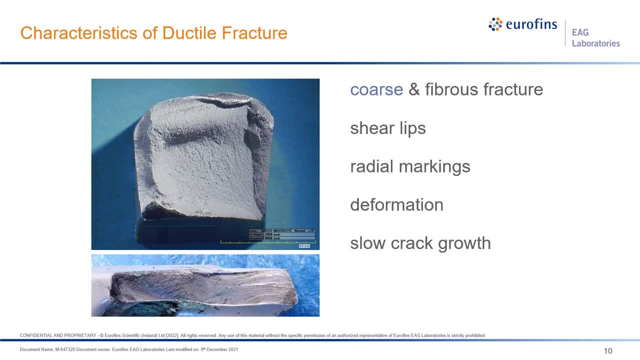 the apex being the point of origin. We also see around the circumference here or around the perimeter. we actually can see this 45-degree shear lip. This is a positive shear lip: it's coming towards us and this is a negative shear. 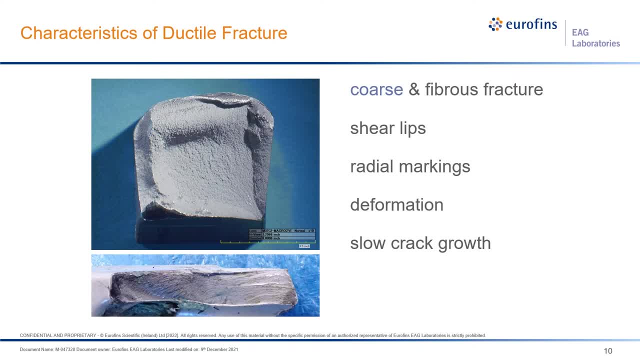 lip: The opposite height, the opposite side of the fracture head. So this is a positive shear lip- It's coming towards us, And this is a negative shear lip: The opposite height, the opposite side of the fracture head. This has, of course, the positive. 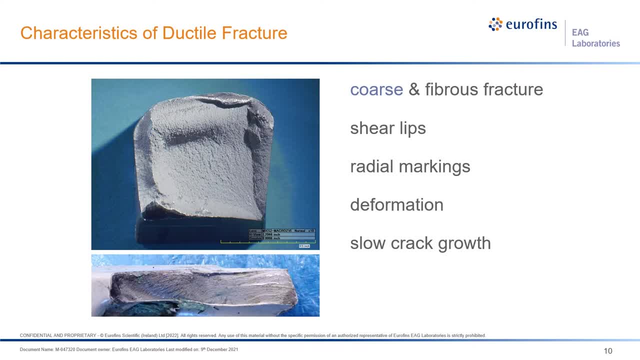 This is metal deformation. Now, in the real world things aren't always this easy to decipher, because in the real world fractures tend to be contaminated, deformed, Sometimes features are obliterated. So we have to obviously deal with what we have, and this is looking at the as received. 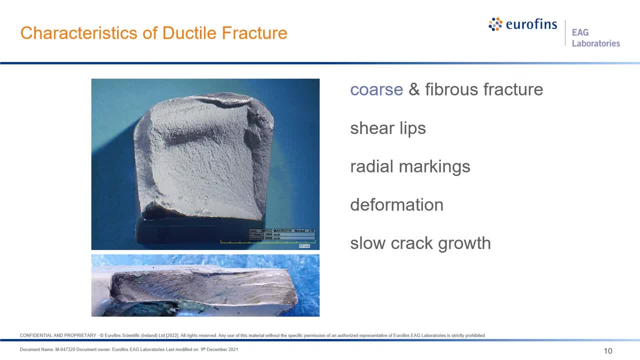 fracture And again follow the action, follow the evidence, follow the lines and we can see a fan-like structure radiating out from down here. So this is all indicating that the point of origin is down here. fractures propagating in this axis. 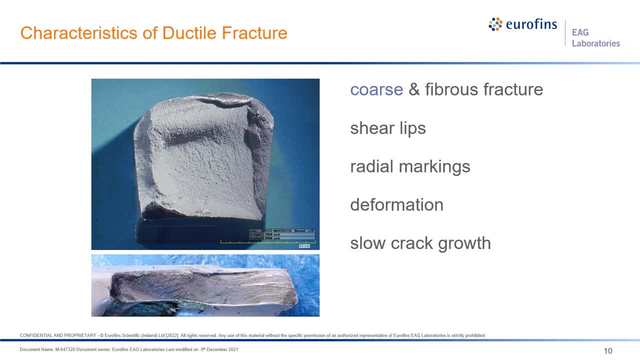 It bent here due to stress redistribution as the fracture proceeded and then tore off, and here's our shearing over here. So this is probably more realistic as to what will be seen in the real world. The markings that radiate out from the point of origin. 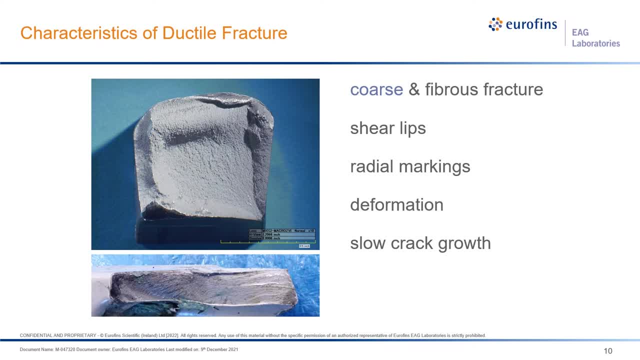 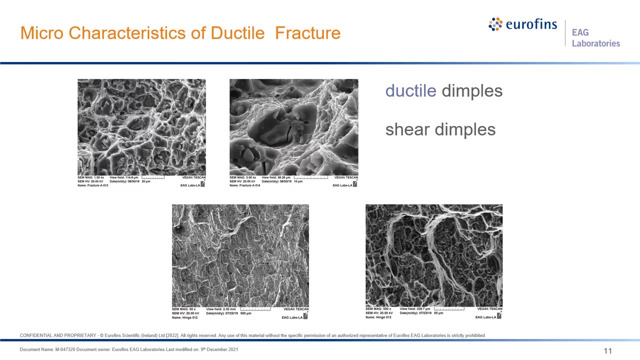 are radial markings. Shear lips, of course, are around the circumference: Deformation. this type of phenomenon, here And again it's a slow crack growth phenomenon. Now, what do we see microscopically? Well, I have to reinforce something here. 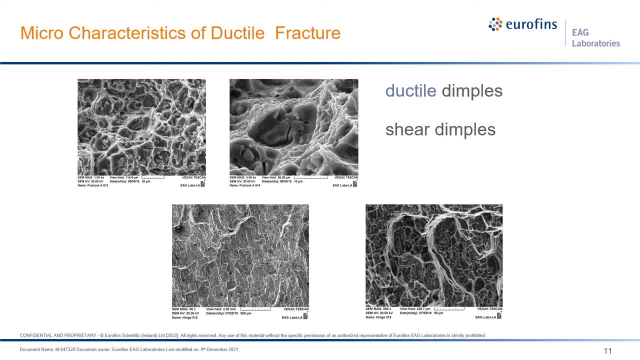 and that is metallography, is crucial to understanding what is happening on a fracture surface. A simple fracture surface, for example iron or steel, will have a simple fracture in ductile. You'll have minute particulates of silicates with beautiful voids that surround them. 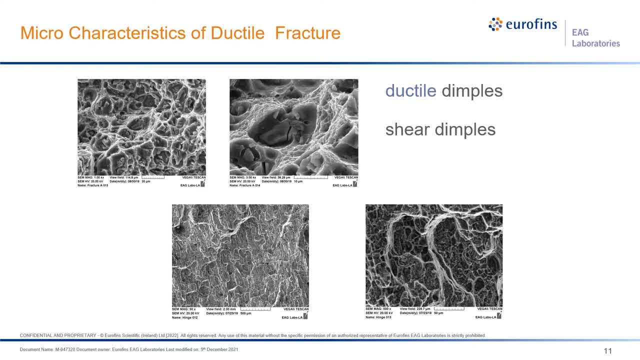 a classic cup and cone fracture, easy to resolve. In the real world, though, alloys are much more complicated- Magnesium alloys, for example. they have an extremely complex microstructure, with a number of different types of particles and phases, all of which are going to manifest themselves. 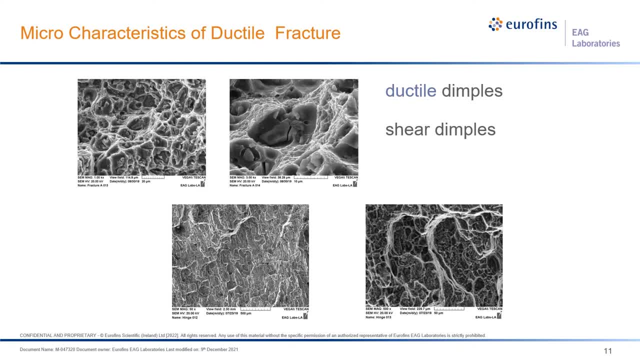 on that fracture surface. So it's important that you understand what you're dealing with before you actually start doing the fractography- unless, of course, you have experience with it. So this is ductile dimples and we can see that the crater 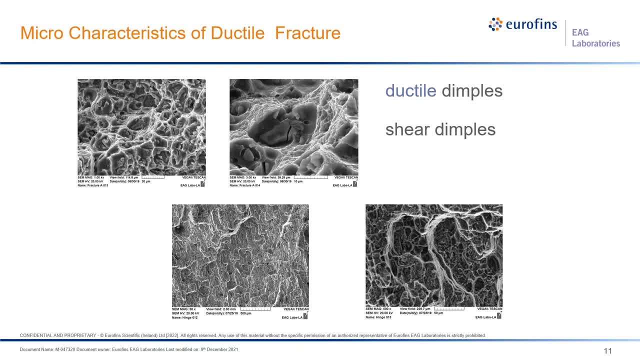 has formed around the particulates And again the crater will form around that particulate and take the shape of that particular particulate. So you have a particulate that looks like a T. you're going to have a T- ductile dimple. 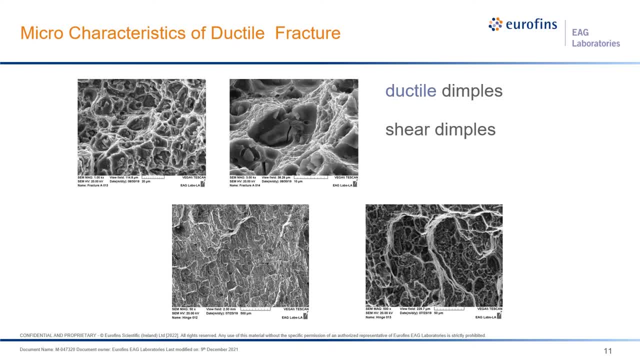 We also see very minute dimples On the wall surrounding, on the crater walls in essence. So here we have very small ductile dimples and here we have the large craters. With the SEM you can also resolve shearing. 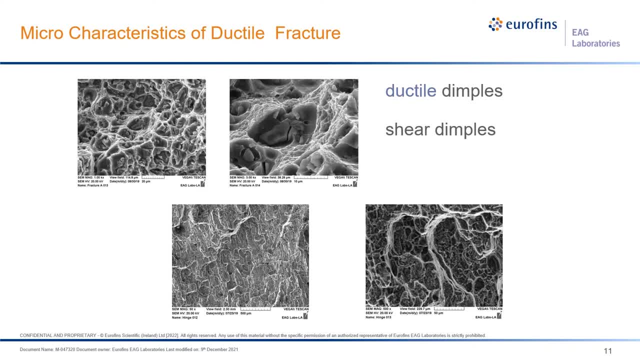 And shear dimples are very important because shear dimples will allow you to determine the direction of crack growth. So shear dimples very important And when resolving shear dimples, the angle at which you resolve them in the SEM. 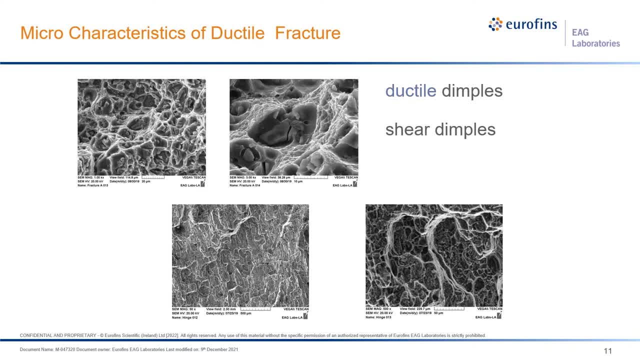 is very important too. If you have the wrong angle when doing fractography, then they won't look like shear dimples. They'll look like equiaxed dimples because you're looking at them head on. But here we can see that we have a shear pattern. 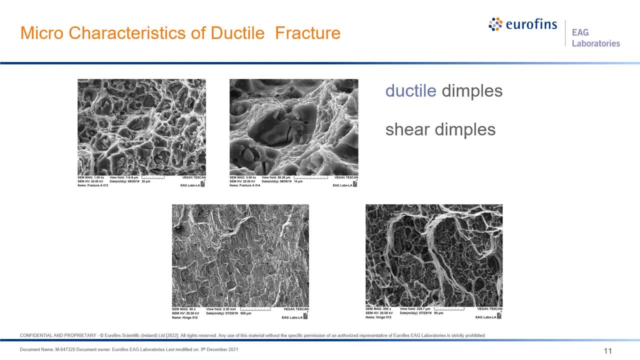 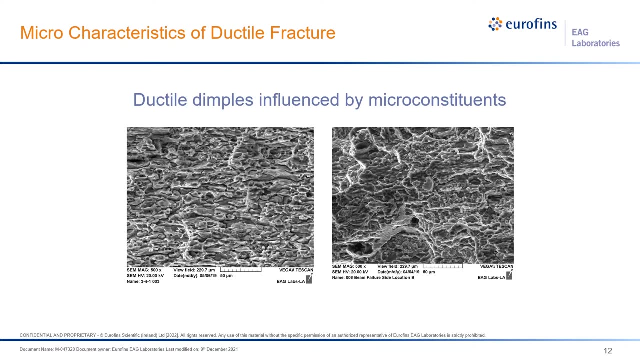 shearing in this axis up here. The angle in the SEM was such that we don't resolve the shear quite as much as we'd probably like to. Sometimes the ductile dimples are influenced by a lot of micro constituents, And here we're looking at a highly worked structure. 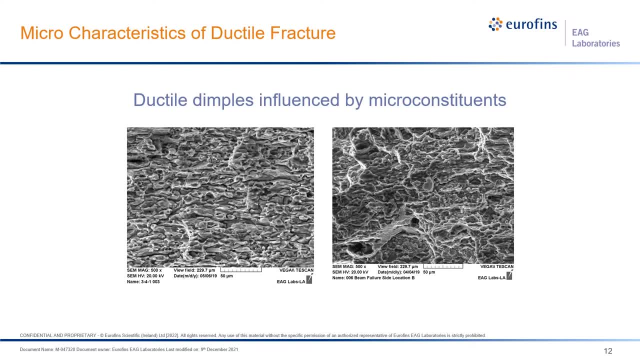 So you can see the bands running in this axis- This would be the longitudinal axis- And then inter-dispersed in, there is all of the parts of the particles that are then forming these ductal dimples. Again, some of these fractures. 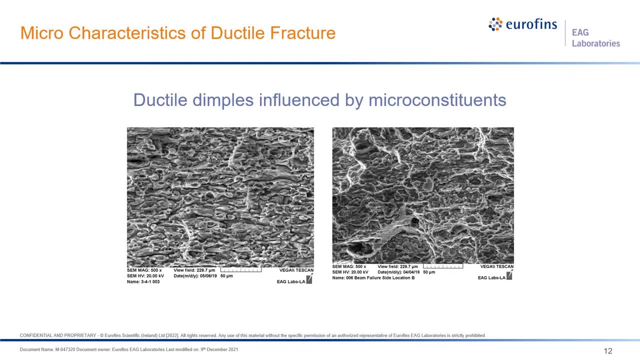 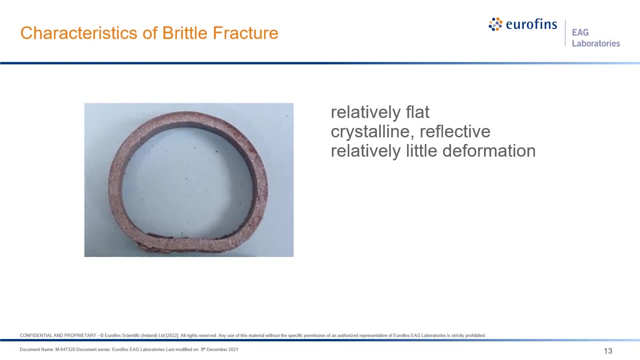 can be very, very busy and confusing. So it is important to take a microsection of the same plane, of the fracture. That way you understand what is going on there. Brittle fracture. simply put, the brittle fracture occurs basically the opposite way. 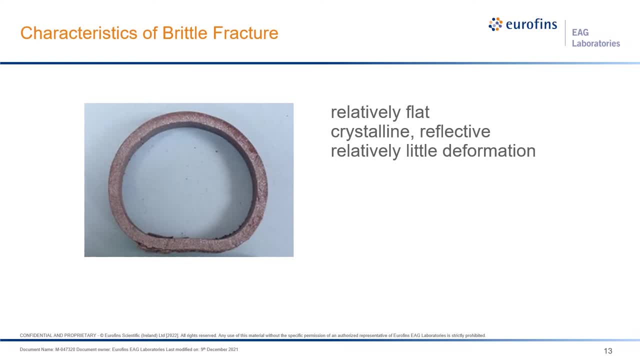 The opposite of with ductal fracture, There is no microvoid coalescence. in brittle fracture You have fracture that is occurring along very distinct crystallographic planes And they are in essence cleaving through those different grains, at different angles, which are dictated by the crystal. 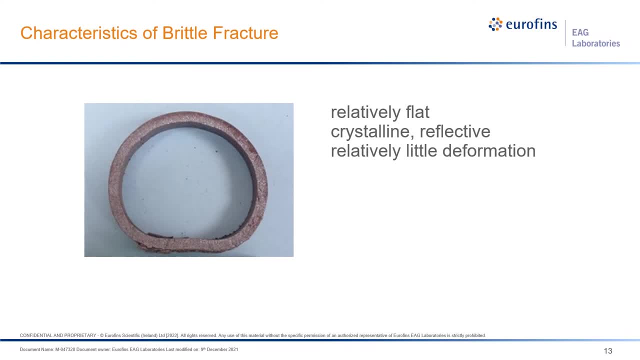 So, macroscopically, when we look at a fracture and we see no deformation, that should be a clue that we're dealing with a brittle fracture. Now, in a perfect world, if this was a classic example of brittle fracture, this would be highly reflective. 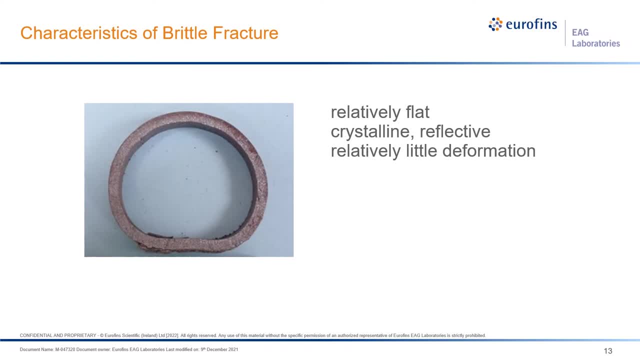 We would actually see a sparkling surface because, even though we're not looking at grains, we're looking at cleavage facets which can look like grains macroscopically. There's no deformation And this type of a fracture tends to be extremely sudden. 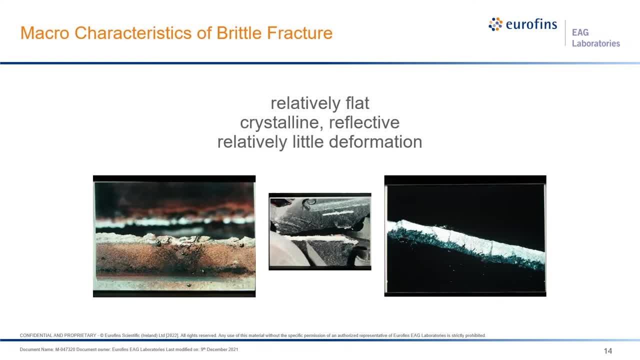 and can be very loud. So, examples of macro features. Well, here's an example of this. by the way, these are features from a locomotive that was accidentally dropped back into the hold of a ship when it was being unloaded. And one of the questions, obviously, 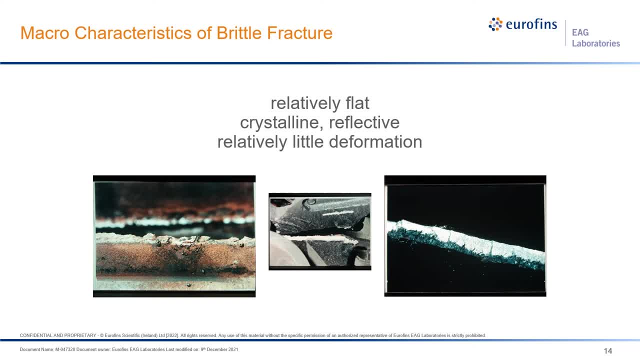 from the insurance company was: was there any thing that was a pre-existing condition that could have exacerbated the damage that was observed? Now, locomotives don't have a suspension per se, So you know they're not. they don't do well when you drop them from two feet. 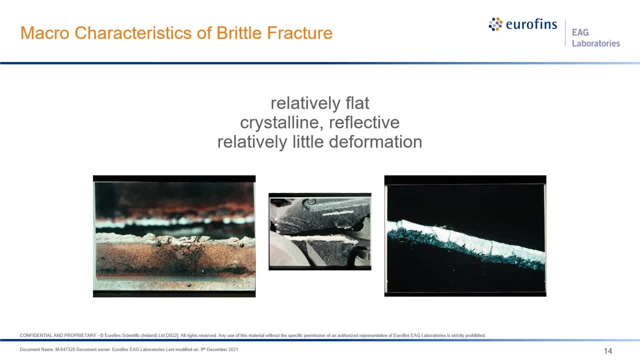 This is a weld in a portion of the locomotive And when looking at this weld, we see that there's no deformation. It's a very brittle fracture. It appears to be flat, And the other thing that's very telling here is it's running right through the center of the weld. 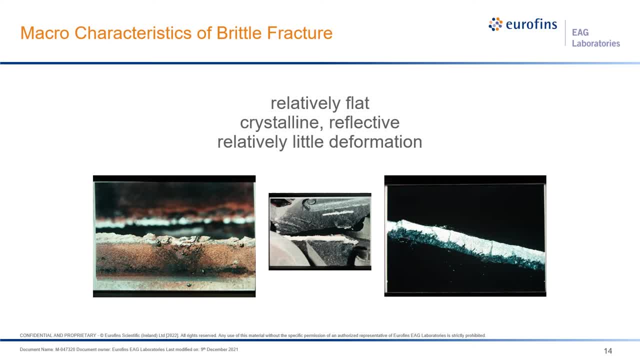 A crack should not propagate through the weld. Normally the weld will be the strongest part of the structure. It should fail in the heat affected zone adjacent to the weld. Well, features like this weld splatter and the charring over here are pretty good indications. 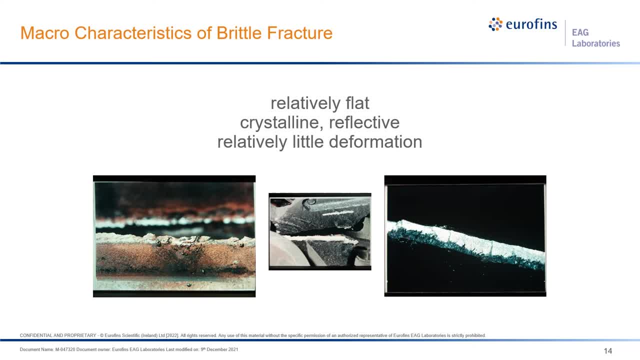 That the welding was out of control. Looking at some of the structure, we see flat fractures but, more interestingly, on that flat fracture we see this black material, which just so happened to be this black material, And, for example, in this segment, 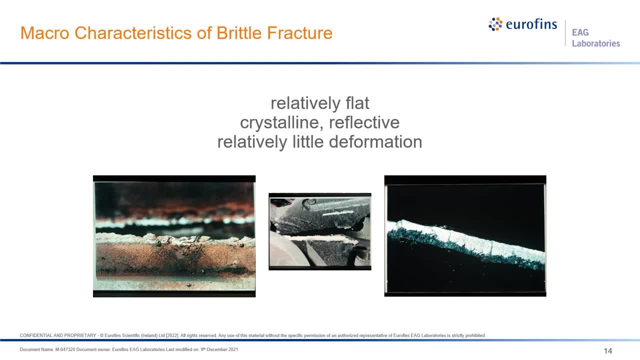 we see that the black material in some areas exceeded 50% of the cross section, which means that that crack was actually there before it left the factory, at least at the time of painting, And then, of course, that served as a pre-notch. 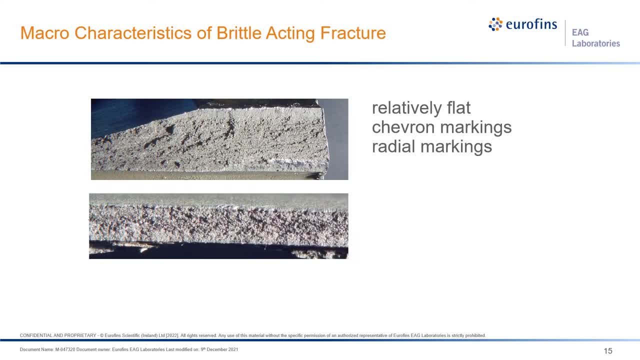 which exacerbated the failure. Some materials, even ductile materials, can act brittle And usually that is because of high strain rates. So, for example, a barrel wall or a pressure vessel that ruptures an explosion Automobile hitting a light stanchion. 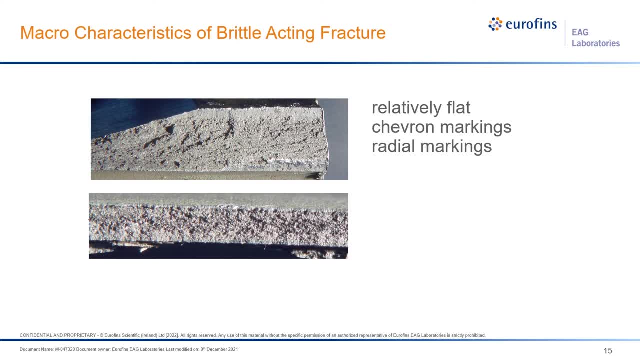 things of that nature. That's fast, that's a very high strain rate fracture And that means that crack is going to propagate very fast And consequently, the fracture doesn't have a chance to rearrange itself, to give you the ductility that would be associated with a ductile material. 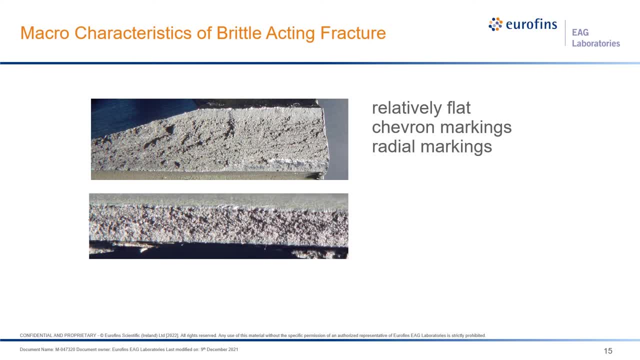 So here we actually see- and again, these are not. this is more like what you'll see in the real world- is you can see a pattern here and that pattern is pointing back to this area. here The pattern is radiating out a bit. 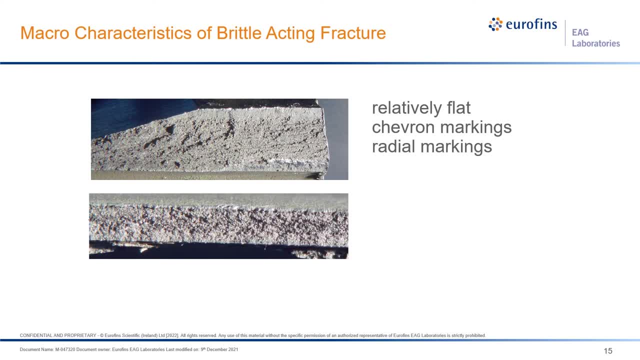 And, more importantly, you have these apexes which are pointing back to the point of origin. Now this is much more evident when we look at it here and hopefully it's a little easier to resolve. We see this recurring pattern. These are the apexes. 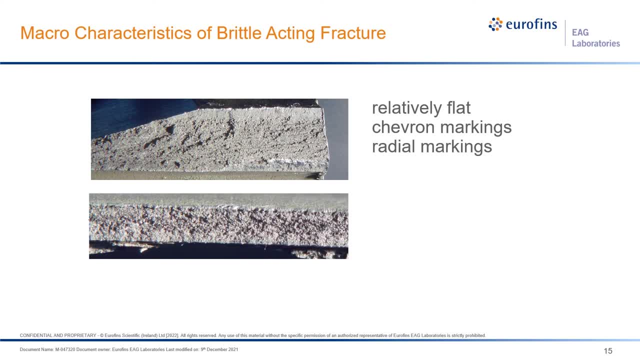 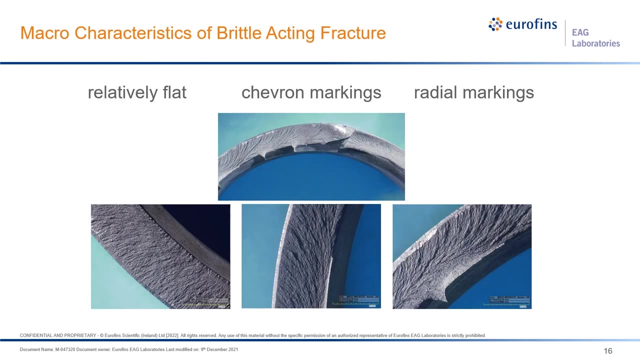 These are called chevron markings or herringbone markings, And these markings are actually pointing back to the point of origin. So the point of origin's over here. The crack propagated very rapidly in this direction. Here's a much better example. 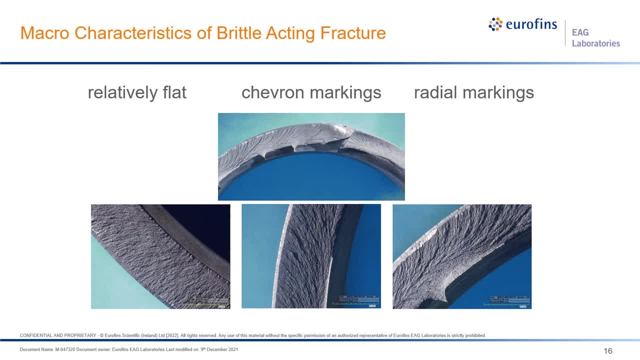 And this is a pipe and what we're seeing is, along the inside diameter, we have evidence of a crack. Now, just to clarify, we can't actually see across the surface of the crack. The crack's obviously a very thin and flat surface. 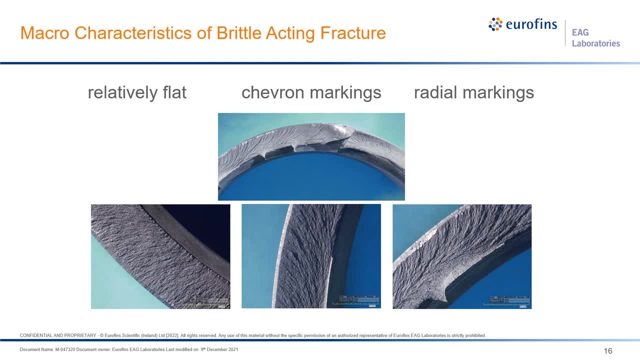 And that's because we basically simply don't have enough applaudation to see where it's going. So it wouldn't be just a glass. It's a surface of fatiguing. okay, It's a very small fatigue region. We'll talk about that in a moment. 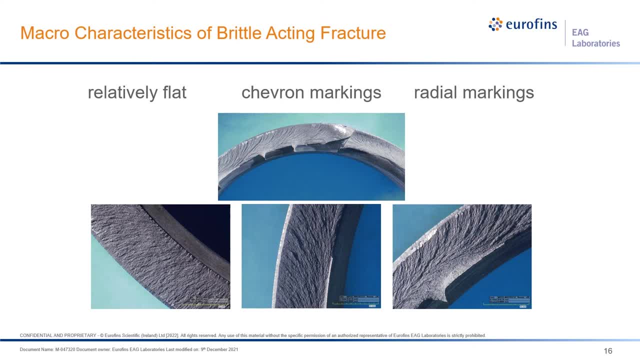 But from that area we have these patterns that are radiating out as the stress redistributes itself, it centers itself, and now we're seeing much more classic chevron markings. where the crack again started down here propagated in this direction. 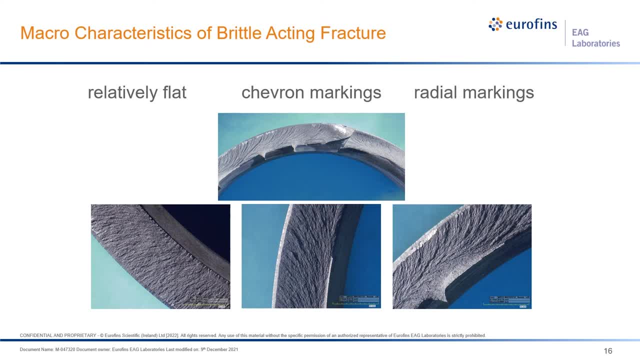 and then at the termination we see radial markings where it radiates out from the last portion of the chevrons. So we can see that the crack propagated in this direction and propagated in this direction and they met on two different levels over here. So 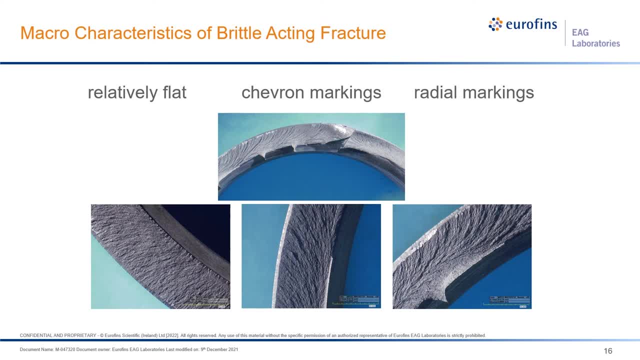 chevron markings are very important for identifying the point of origin and the point of final separation, and they're extremely important when dealing with highly complex failures such as an explosion or an exploded pressure vessel, because it seems daunting when you have all those broken pieces to examine. 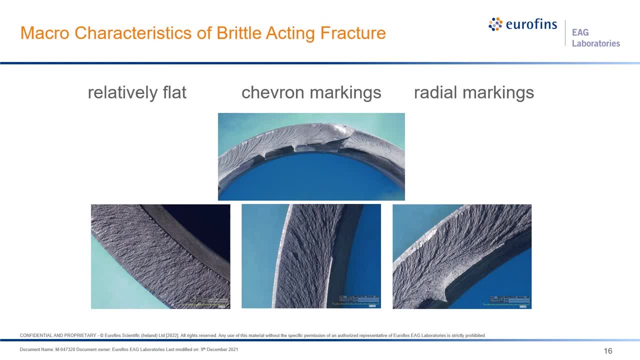 But if you see the chevron markings on there and you see these radial markings, it's very easy, well, relatively, to examine each segment and if there are chevron markings from one end to the other, you can discount that sample because your origin is not there. 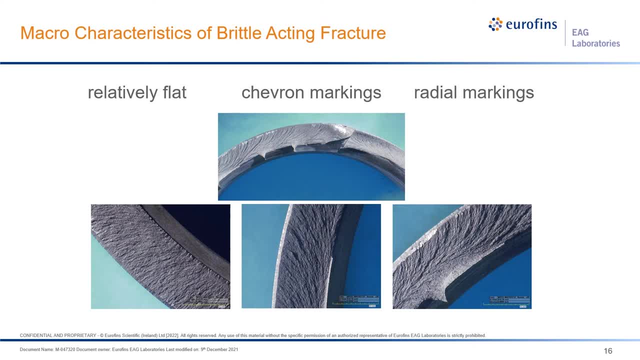 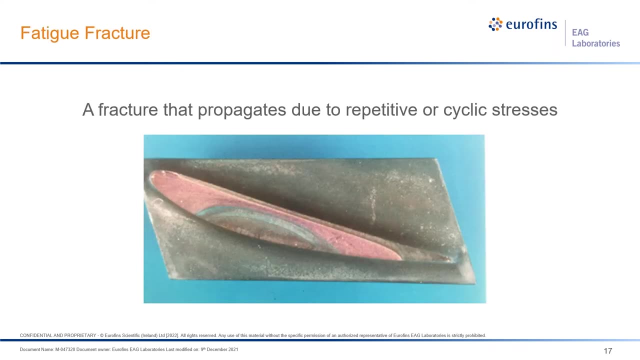 and you move along until you find an area where chevron markings converge and that will be your point of origin. So they're very useful And, of course, chevron markings can be used to map out how that fracture propagated. Now fatigue. 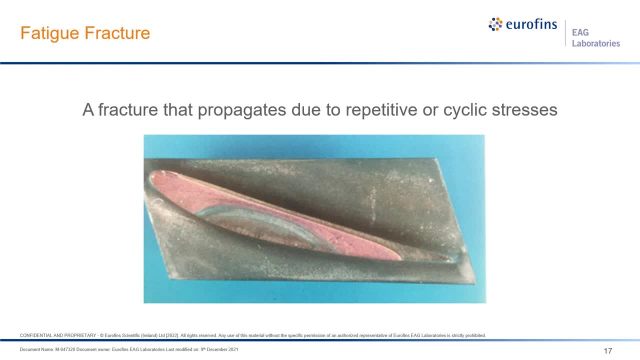 Many, many failures occur in fatigue, and fatigue is a fracture that propagates due to cyclic or repetitive stresses, and these stresses are below the tensile strength Okay. So fatigue can be insidious. You can have a fatigue crack propagated. 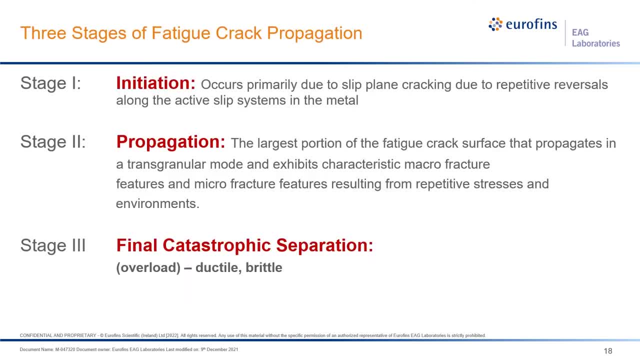 You can have a fatigue crack propagating and you don't even know it. How can that be? Well, we'll talk about it in a moment. Stage one, fatigue, is the initiation, and a great deal of time is consumed in that initiation process. 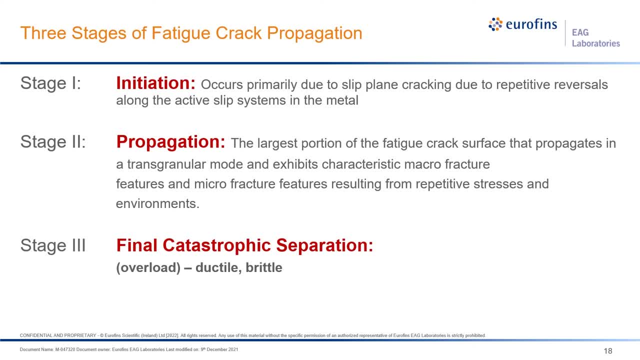 and that is occurring along slip planes. This cannot be observed and consequently, for example, a turbine blade can have stage one initiation, It can be overhauled, It can be put into service and as soon as it's put into service, go into stage two. 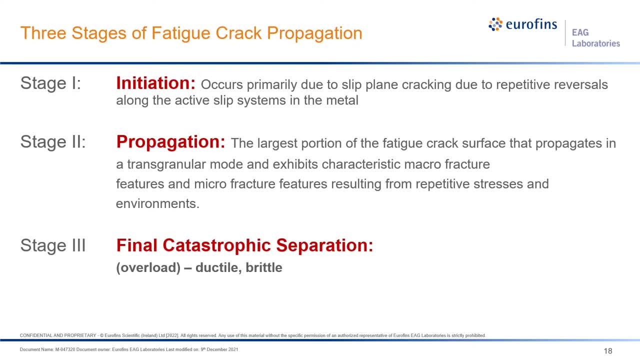 which is the crack growth period, and then fail. So fatigue can be a bit insidious. So we have initiation, We have propagation, which is the largest portion of the fatigue crack growth, and then we have final catastrophic separation, which is going to be either ductile or brittle. 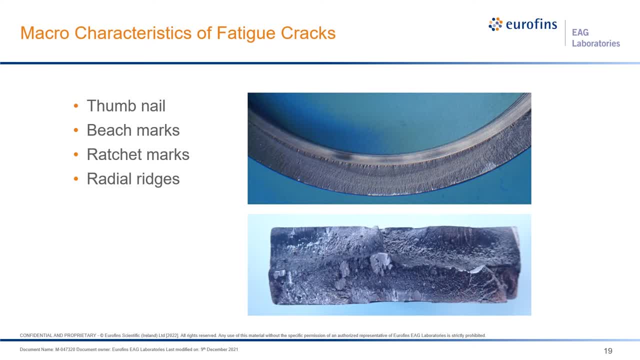 So one of the telltale signs Of fatigue is something called a thumbnail, and a thumbnail indication is a large flat region, And you know. so you have a coarse morphology, and then you have a large flat region that tends to, you know, be concentric. 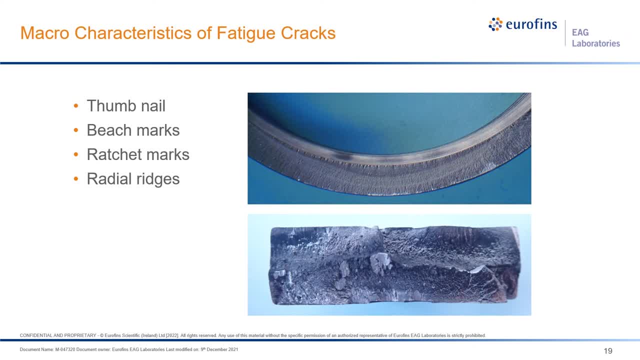 In this instance, we have this large fatigue thumbnail and that indicates that the crack started here and propagated out in this direction. It radiates out. It radiates out from this edge and then we have secondary thumbnails at the backside, which indicates that as this crack was growing, it started to bend and put the stress on the backside. 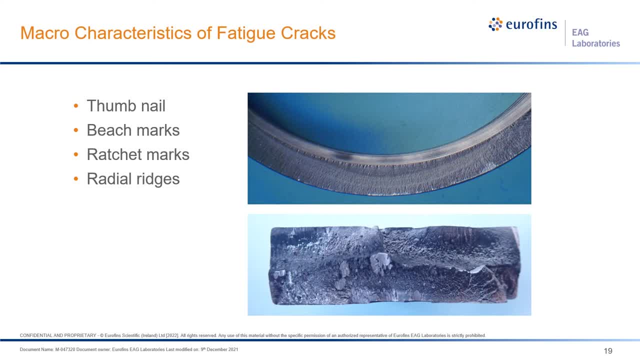 which initiated a fracture here and another one over here. The largest and deepest of these thumbnails will be your initiation or your primary. Here we have a situation where we have a small thumbnail which is darker and then we have a larger area and a larger area, and we can see that this actually propagated all the way through. 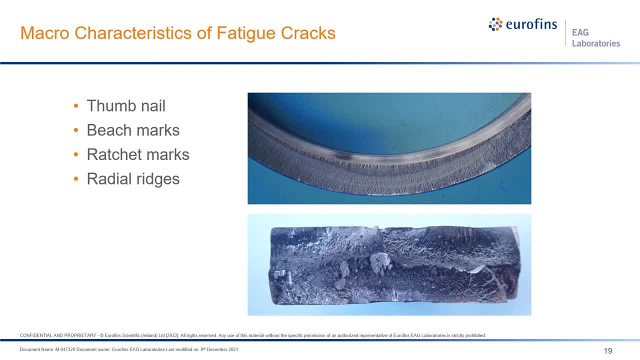 And we see these different colored bands. Those bands are your beach marks and those beach marks indicate different periods of crack growth Along the edge. here we have these small features, the V-shape features that are called ratchet markings, and they are indicating where the point of origin is. 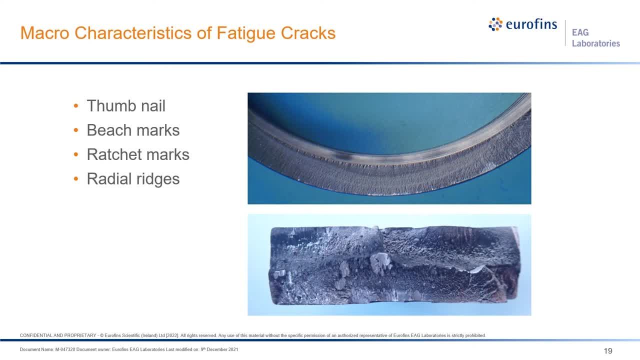 and they are indicating where the point of origin is was. In this case, you have multiple origins, but the primary being in the center of the deepest portion of that thumbnail, And then, once the crack separates, then you have radial ridges where the 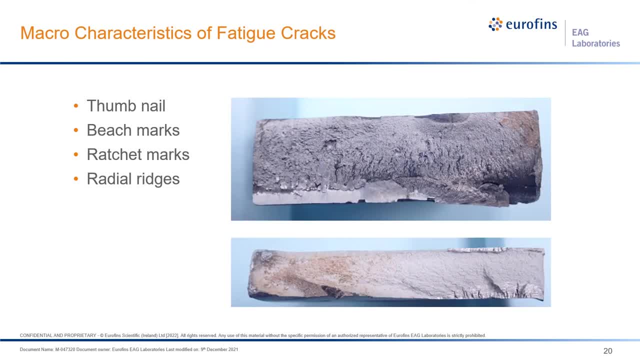 crack radiates out in overload. So here's some very nice examples of a thumbnail. When the entire surface is very coarse and fibrous, obviously there's a lot of ductility here. but lo and behold, you see this small concentric region here, And we have two. It looks like there's this one and then 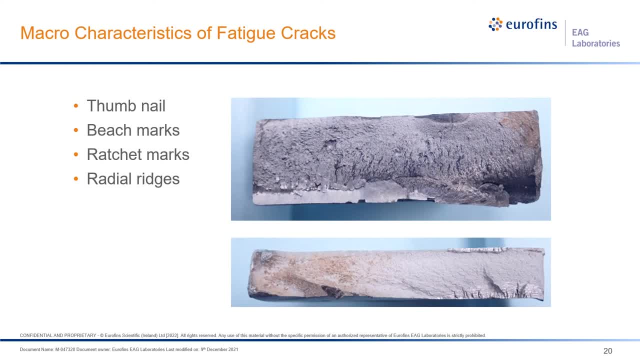 there's this one. Well, it's the same fatigue fracture, but this one appears to have been there longer and may have propagated and then arrested. Maybe the part was taken out of service for a while and then it was put back into service and it propagated some more until it finally went. 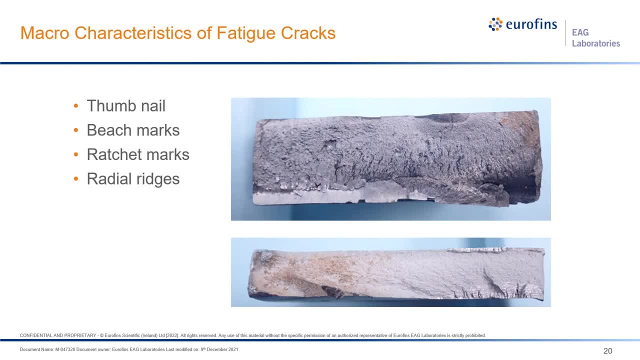 into overload and final separation. Down here again, we see these radiating marks that allow us to see the direction of crack propagation. We have the apex down in here, which is where this flat, shiny surface- again, that's your fatigue thumbnail. Here's your very pronounced ratchet marks in between these Vs. That's your 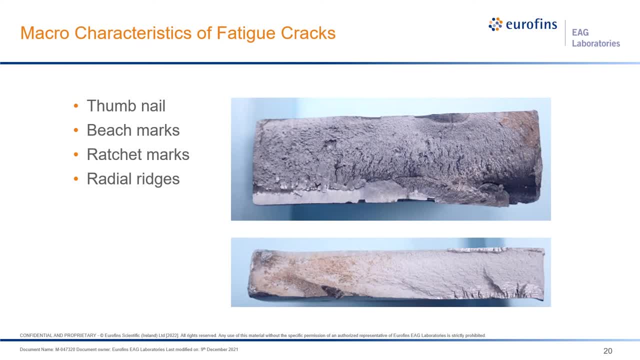 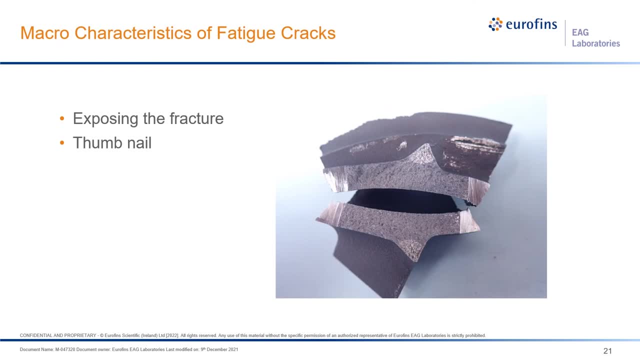 point of origin there And the primary point of origin is going to be opposite, the deepest portion of the fatigue. Now, in a perfect world the samples would come to us ready to examine and nice and clean. But in the real world oftentimes we're presented with a component where there's a minute hairline fracture that was identified with. 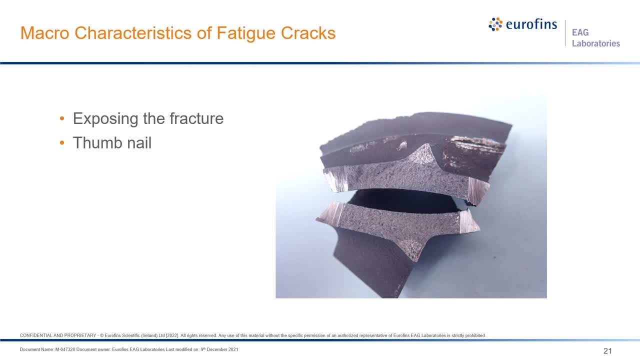 non-destructive testing, perhaps dipenetrant. We need to open it so that we can actually see that fracture. And there's a number of procedures that you can apply to fracture opening and they all depend on the sample geometry configuration, how deep the crack propagated. But basically what you're. 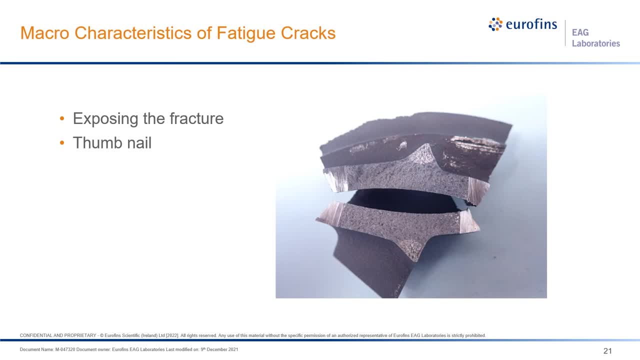 doing is pulling the two halves of the fracture apart, And some materials can be deceivingly strong. Many a technician has ended up on the floor from trying to do a tug-of-war, opening up the fractures. But here, once we open the fracture, we see a very nice small reflective thumbnail. 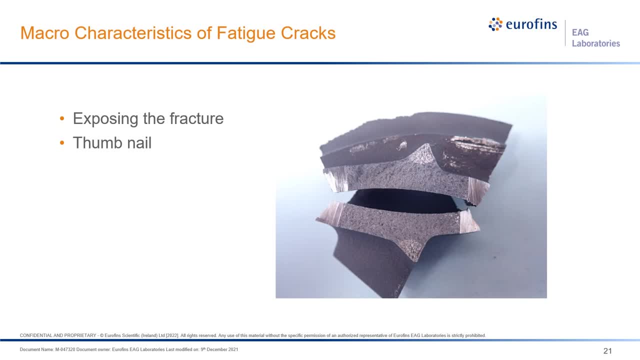 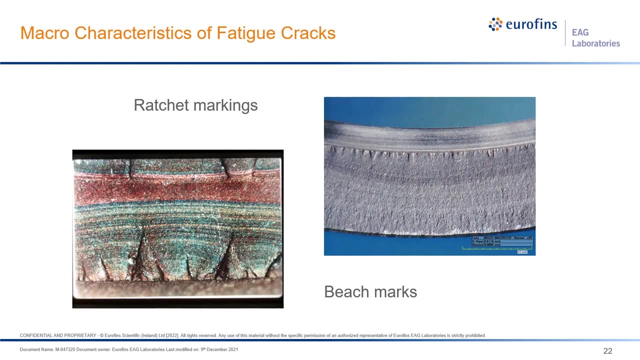 So this would be then where we concentrate our analyses, and it all propagates out from here. Okay, And again ratchet marks and beach marks, Some cases, for example this turbine blade failure. we have beautiful examples of both. We see gorgeous examples of ratchet marks. 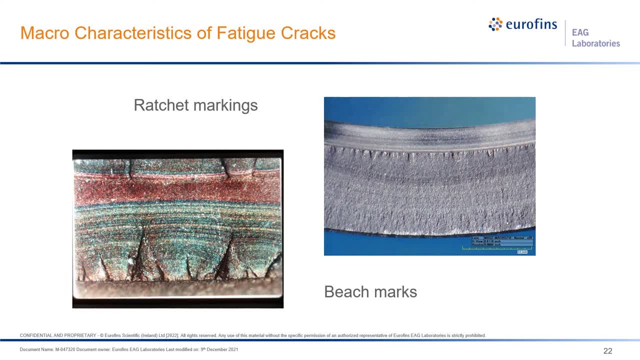 If we look down in here, between these two ratchet marks we see smaller ratchet marks And in some cases you would actually see a tiny thumbnail. So you would see a thumbnail that propagates and the fatigue starts to grow along this plane. 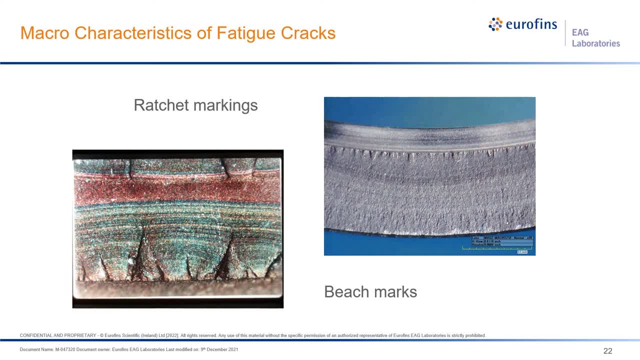 Meanwhile, another fatigue crack starts to propagate along this plane, And another one along this plane, And it starts to propagate over here and over here And eventually all of these fatigue- basically fracture marks, coalesce together and form one advancing crack front. 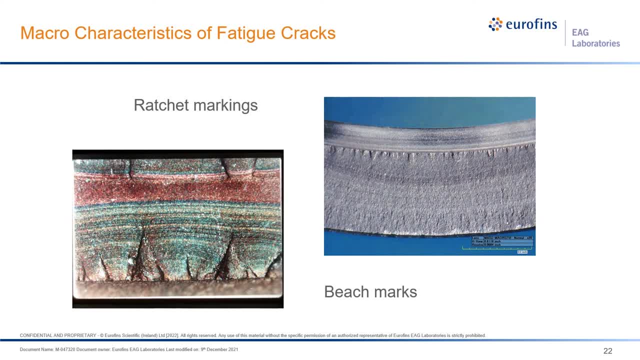 Okay, Well, you notice that these individual beach markings have different colorations. These are not to be confused with fatigue striations, Which indicate one load cycle. You can have millions of fatigue fracture striations within an area of beach marks. These are a little narrow, so I don't think you have millions, but certainly you'll have thousands. 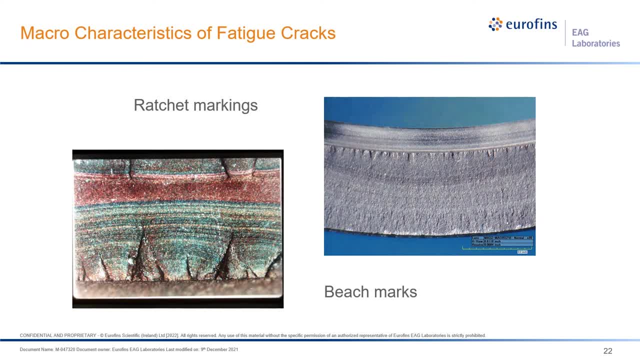 And what you will see here is each one of these bands indicates a different period of crack growth under different conditions. So these were formed by differences in the loading occurring And the loading occurred by the engine. So different periods of the engine cycling, the amount of thrust, et cetera, is being reflected on the surface here. 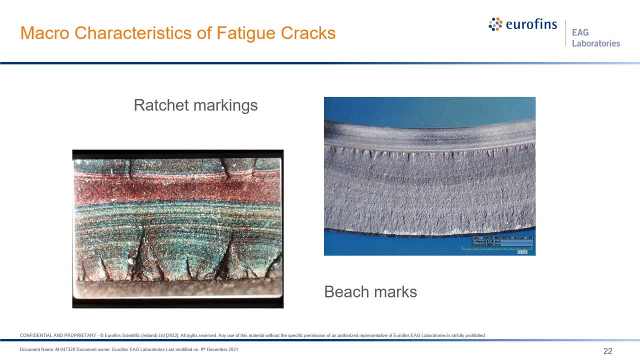 Well, as the crack propagated through from the high-pressure side towards the low-pressure side. we see another beach mark, Very nice thumbnail here on the backside. And so once the blade thickened, Once the blade thickness was compromised, then the blade starts to flutter. 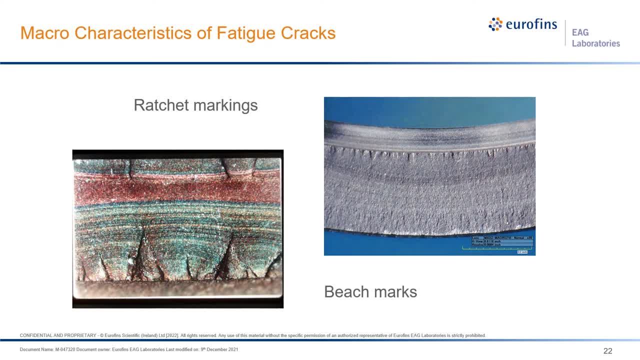 And stress is applied on the backside, A secondary crack starts to propagate in And final separation occurs here. This is called reverse bending loading. Another example, And I'll move right along here, And this is again. you see your ratchet marks. 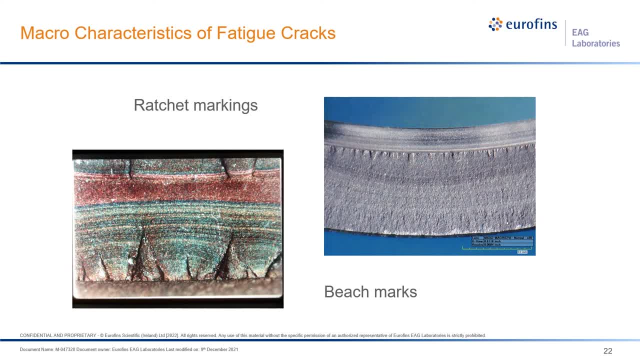 You have a beautiful dark fracture region here. Perhaps the part was taken out of service for a while And then allowed to propagate And you do see differences in textures. And again, those differences in textures indicate differences in load amplitude, environmental conditions and atmospheric conditions. 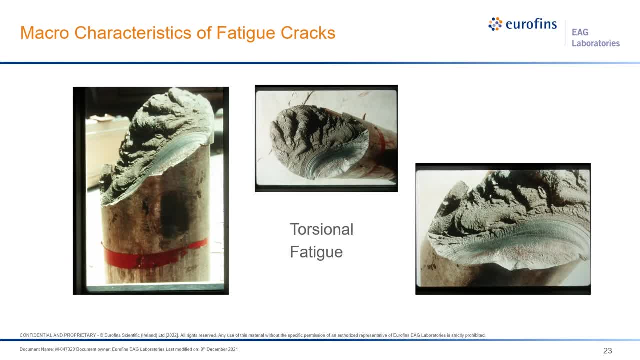 Now, this is a gorgeous fracture, if you like fractures, Because now what we have is a perfect example of torsional loading, And we can see when there is a fracture that is broken, A fracture that is at 45 degrees to the long axis. 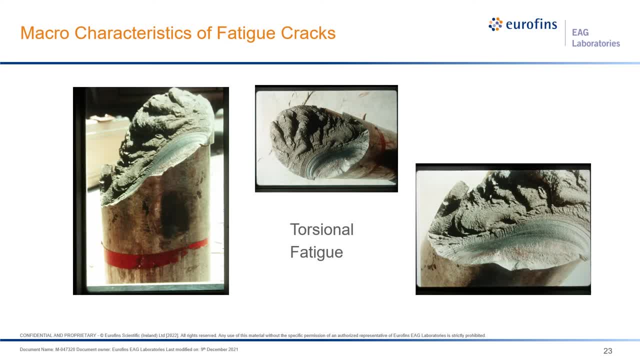 Then that is a dead giveaway that we have a torsional load. So when we look down on that shaft again, we see the ratchet marks here, We see the beach marks propagating out, And then we see all this ductility. 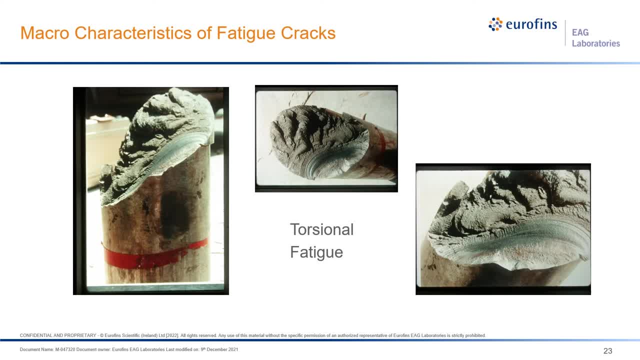 A lot of ductility. I mean look at all that deformation. So a very ductile material. But in spite of how ductile it is, Look at how flat that fatigue fracture is. And again, 45 degrees indicates torsion. 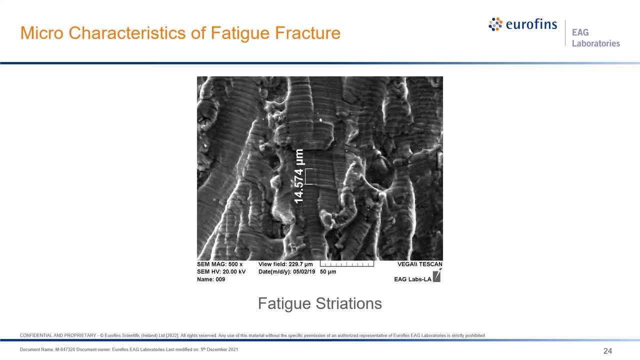 So what do we see at the microscopic level? Well, in the real world, this isn't what you see. In the real world you see smearing dirt, contamination threads, Anything but beautiful fatigue striations. Sometimes you're lucky to find four or five of them. 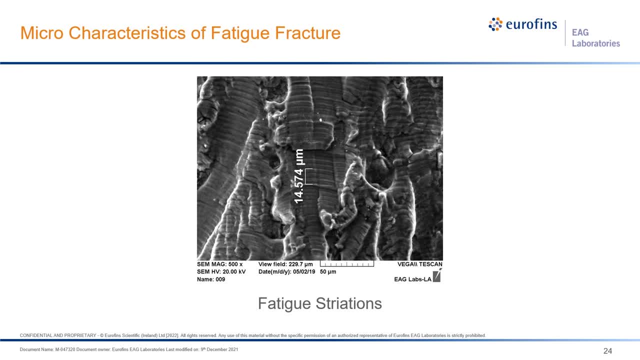 But in this instance We got lucky And we have beautiful striations And each one of these is a period of crack growth from one cycle of crack growth. So each one of these is one crack growth cycle and a rest during stage two. 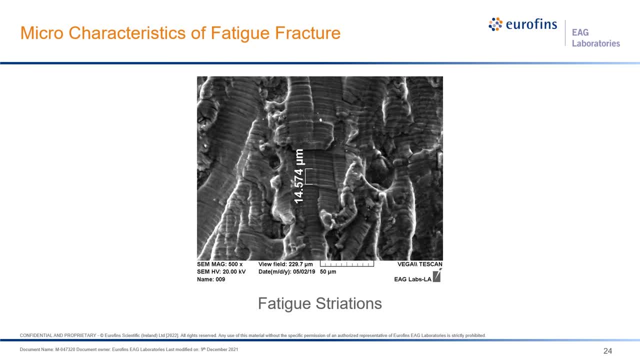 Which is the propagation stage, And we can see it's very prominent along one plane, Another plane over here, But they are all prominent And they're propagating in the same direction. Now, when there are no obvious fatigue indications, striations, 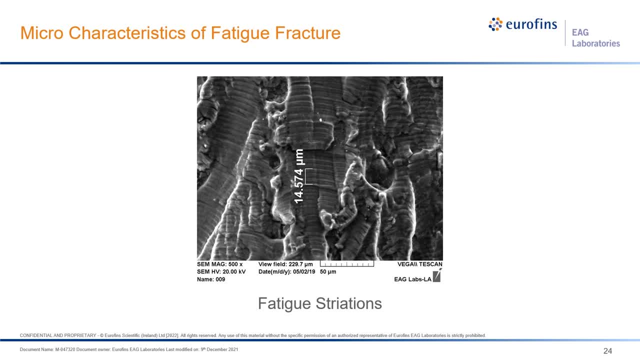 The place to look for them is right next to ridges or in low spots, And sometimes you'll be able to see some, Because remember that a fatigue crack propagates by opening and closing And oftentimes obliterates itself During crack growth. 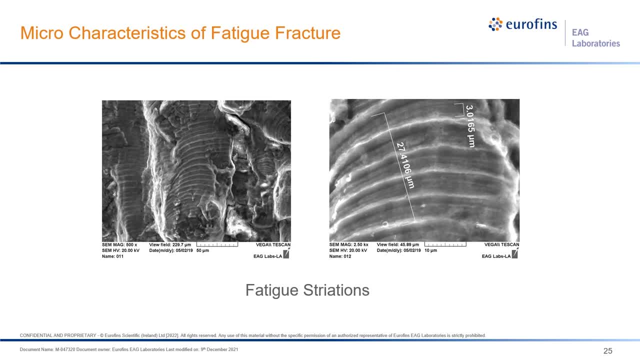 Another thing I'd like to caution is when looking at fatigue fracture, It's important that you exceed the magnification at which you initially observed the striations Here. we look at these striations and we say, aha, We have striations. one load cycle. 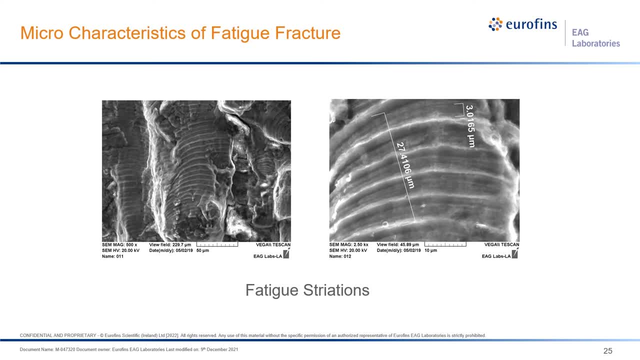 But you need to go higher Because oftentimes you'll see secondary striations. So there's two types of loading going on here. Perhaps these large striations are from the flexing of an aircraft wing And the small striations are due to something like the vibration from the engine. 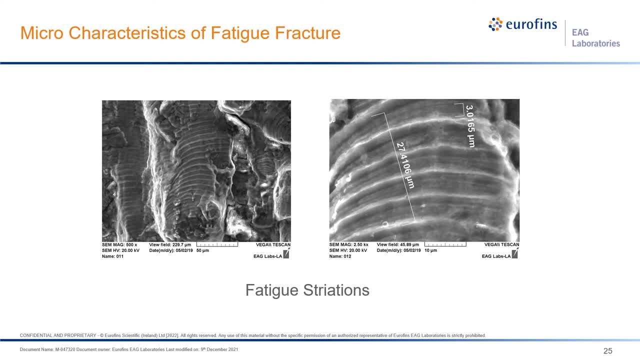 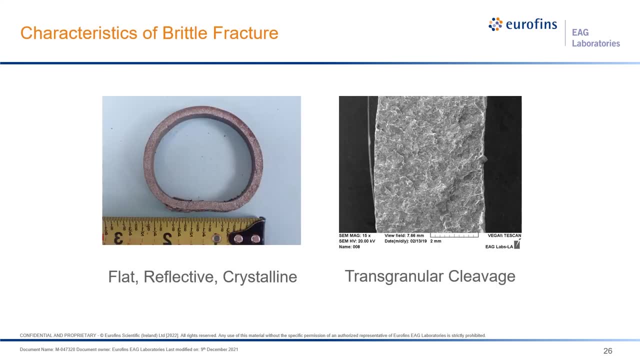 So it's important to exceed the magnification of the initial striation. Okay, brittle fracture, Brittle, flat, reflective and crystalline And transgranular, crystalline, Transgranular cleavage. So we see it's flat. 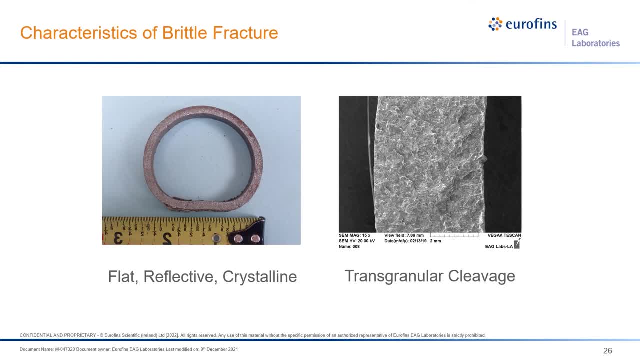 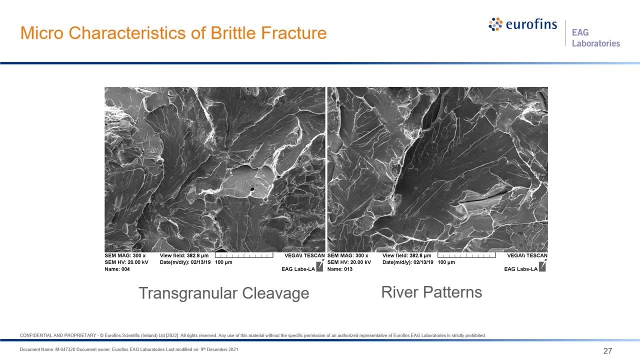 If it was a color image, we'd see that it was reflective, And when we look at it at higher magnification, we can see these cleavage planes Very pronounced. We have a cleavage facet here, Another one here, Another one here. 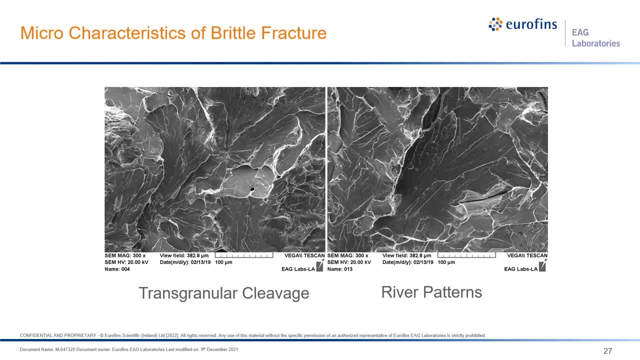 This beautiful large cleavage facet here, Another one over here, And these marks, This little wishbone down here, These are river markings. These are all river markings And they are basically telling you the direction of crack growth. So with brittle fractures sometimes you do not have radial ridges or other features that will indicate the point of origin. 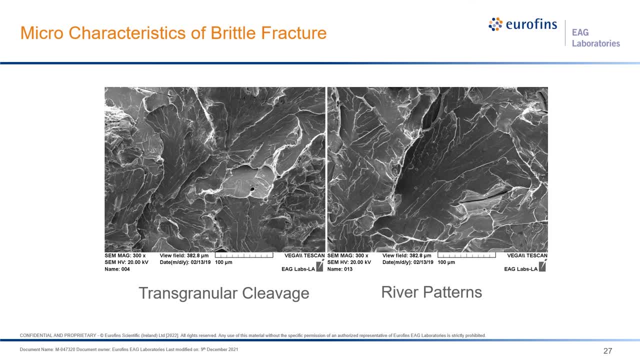 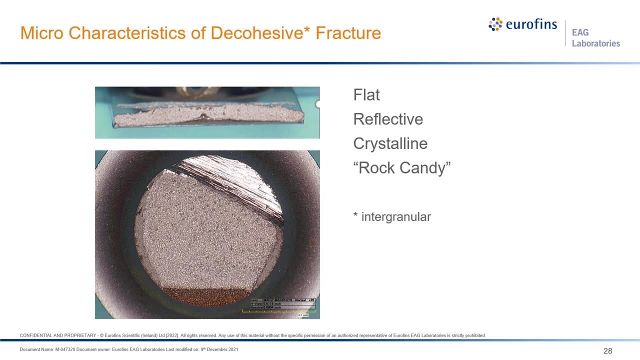 But by studying the fractures and looking at the features on the cleavage one can determine the direction of that crack growth. Decohesive. Decohesive fracture is intergranular fracture And that indicates that something went horribly wrong because the grain boundaries, basically, were weakened to the point of separating. 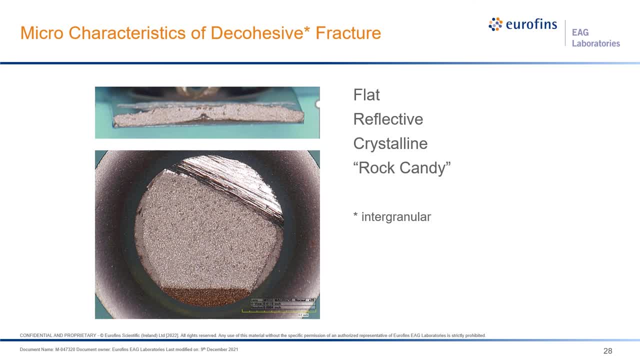 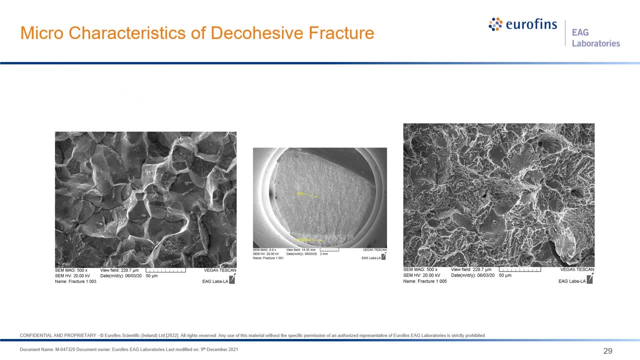 And one of the most insidious causes of this type of fracture is something called hydrogen embrittlement. Where hydrogen is introduced, it remains dormant until a stress is applied, And then this is what you get, And here we see grains. These are not cleavage facets. 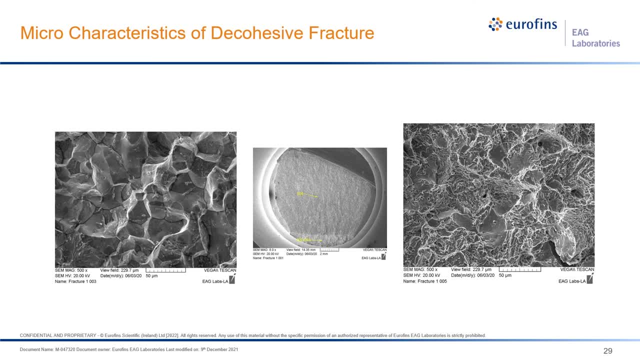 These are actual grains And we see that the crack is propagating along the grain boundaries. We have secondary cracks that propagated from the primary And in this region over here, this was that darker region, Here's a lighter region And we see that the hydrogen intruded along this edge over here. 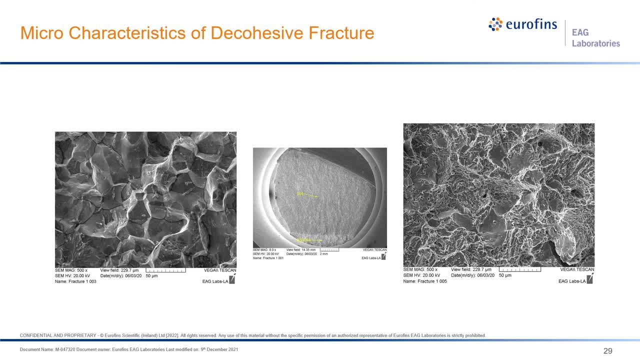 And out here there is some brittleness from intergranular, So there was some hydrogen, But for the most part we're seeing ductility Okay. So this is confirming that we had a ductile material to begin with that became a brittle one due to hydrogen fracture. 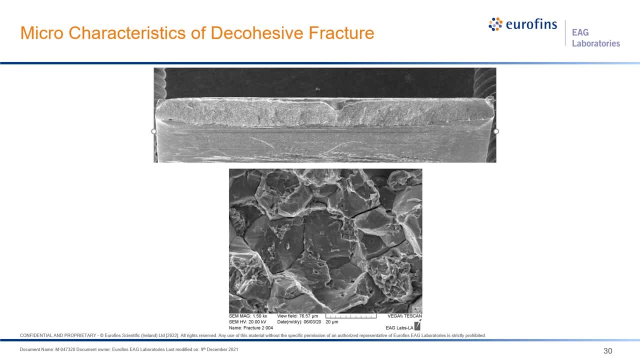 A fastener that fractured And again we see the rock candy appearance. But here we're seeing some ductility. We actually see some ductility on the grain boundaries And we see some small features over here. These are basically crow's feet. 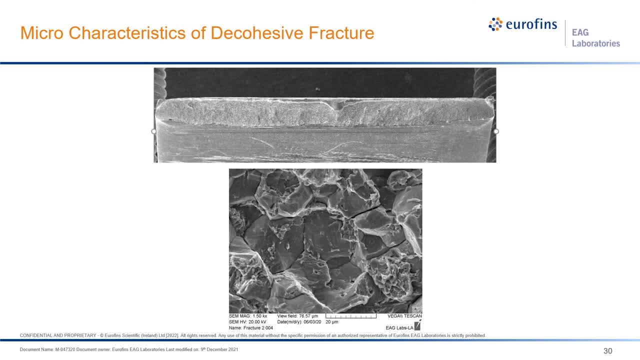 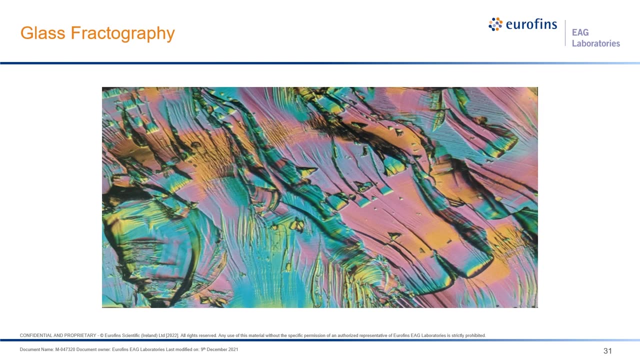 And these are all features that will help you confirm that you're dealing with a hydrogen fracture, as opposed to stress, corrosion or some other mechanism. And, last but not least, this beautiful image is actually a piece of quartz And we were asked to do fractography on it. critical application. 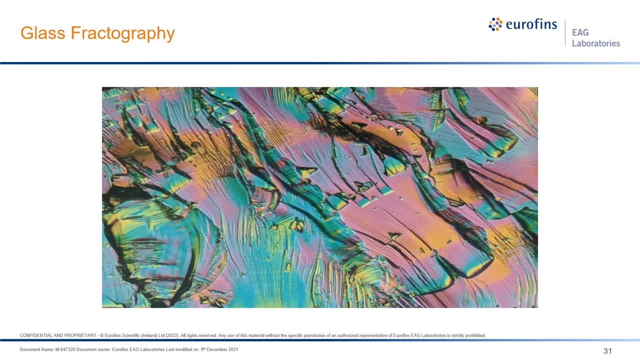 Unfortunately, it's difficult to see fracture features on quartz, But using polarized lighting techniques, we were able to very nicely resolve all of the different fracture features. And the nomenclature that we discussed today were steels and metals. Okay, So the fact that we have steels and metals is completely different for glass. 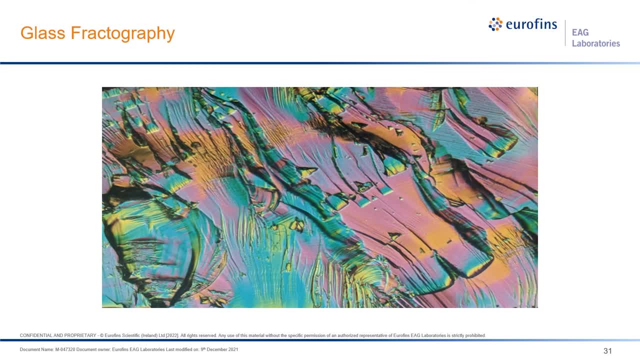 I mean for glass fracture. we have terms like mist, hackles, things of that nature, But the mechanism is very often the same. Additionally, fractography can be applied to nonmetals, composites and other engineered materials, ceramics, et cetera. 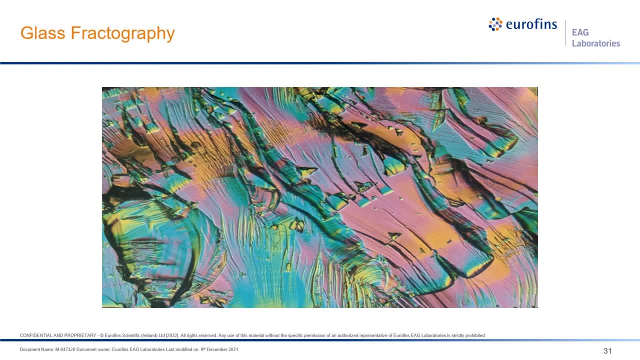 We have some highly qualified people that can address that. We have some highly qualified people that can address fracturing in polymers. So if there's a pattern on it, chances are there's a way to read it and use it. So what do we do?